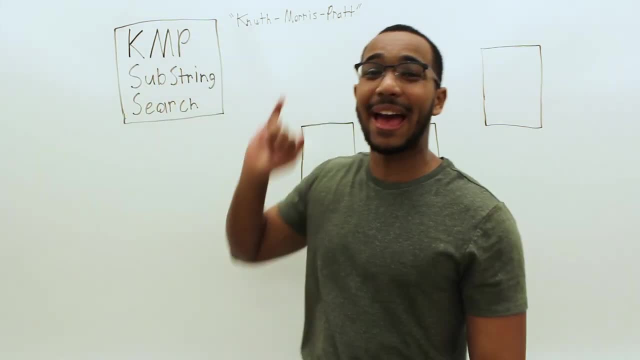 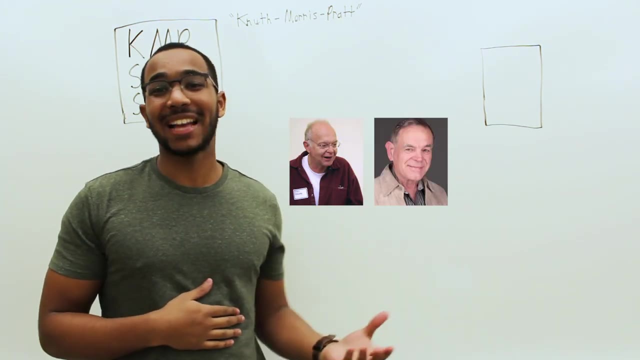 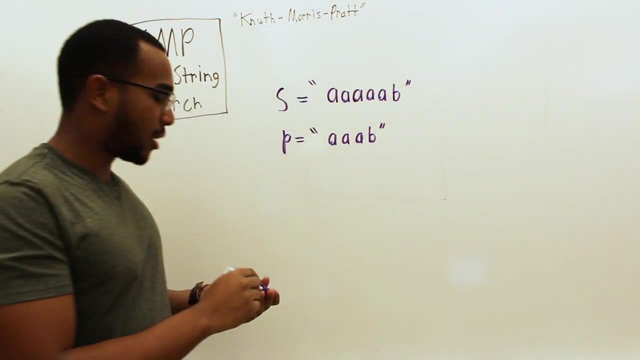 Alright, so today we are going to talk about a topic called KMP substring search. This is an algorithm invented by Donald Knuth von Pratt and, independently, by a third guy named James Morris. So basically, what the whole point of the algorithm is is we're given a pattern and we're given a string. 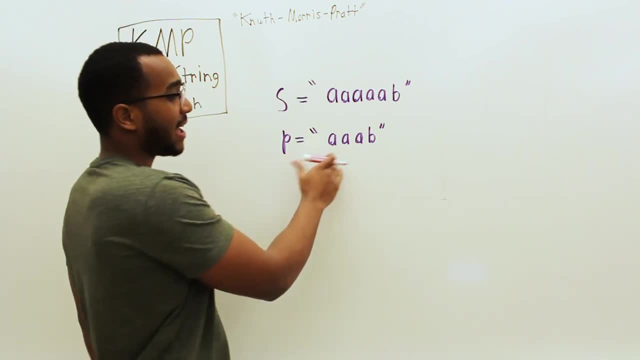 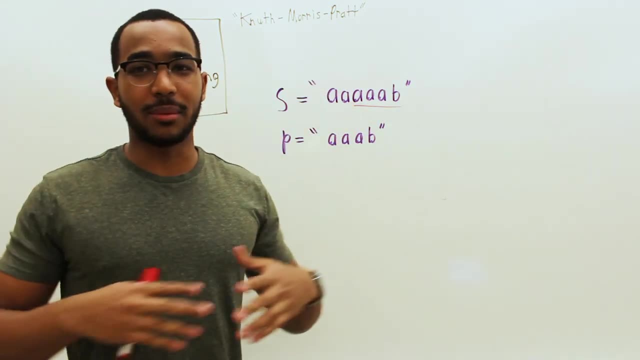 And our goal is to find whether the pattern exists in the string. We see that AAAB exists here in the string. So the whole point is we want to find this indice and return that value- or it could be different variations of that, But the whole point is find the pattern in the string. 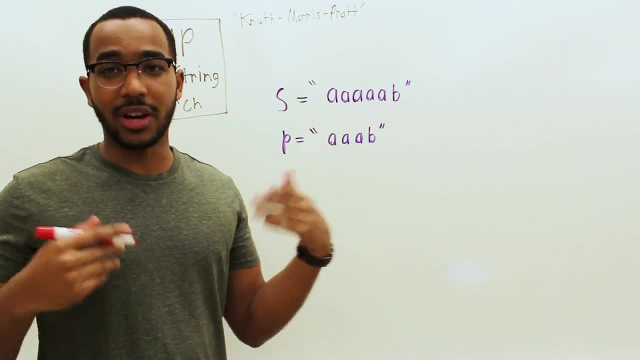 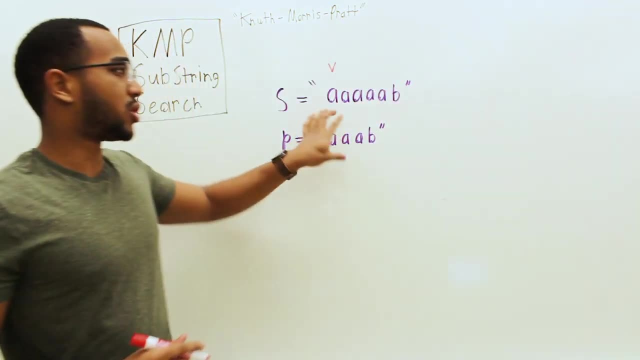 What we do is the normal way that it's done. the naive approach is to look at the first characters. These match. So because these match, we're going to begin a search on A. So these A's match, So they match. so move on to the next characters. 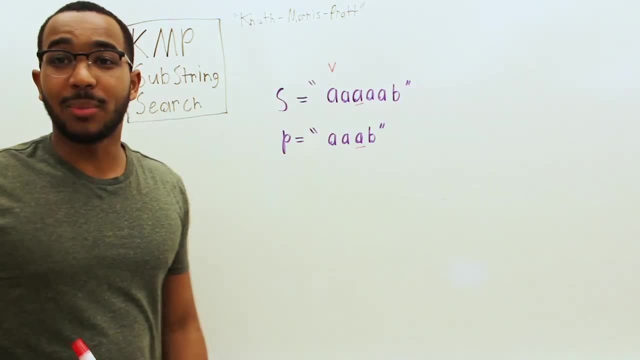 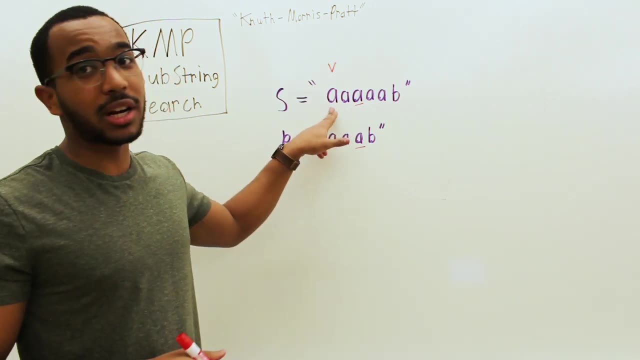 Do those match? Yes, Advance forward. 1.. Do those match? Yes, Advance forward. 1.. And notice, we're still doing a search, just on A. We're just saying if this substring started here, is it a match. 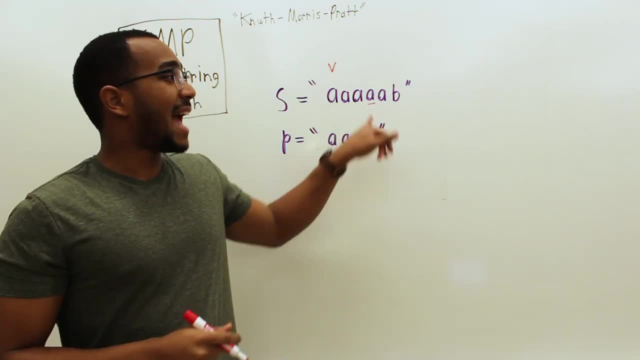 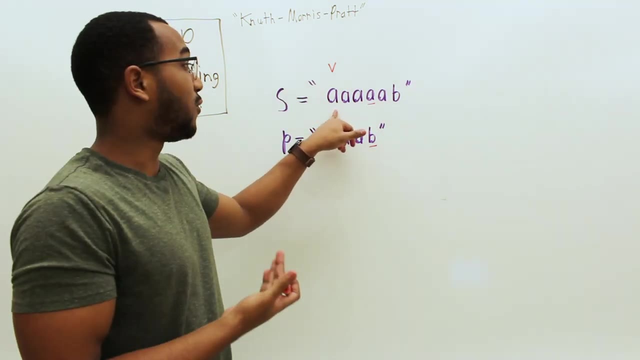 So advance 1.. And what we see is: A and B do not match. So our substring pattern one it does not exist. It does not exist from this indice. So therefore, we advance forward 1 from here. And so we check: Do A and A match? Yes, they do. 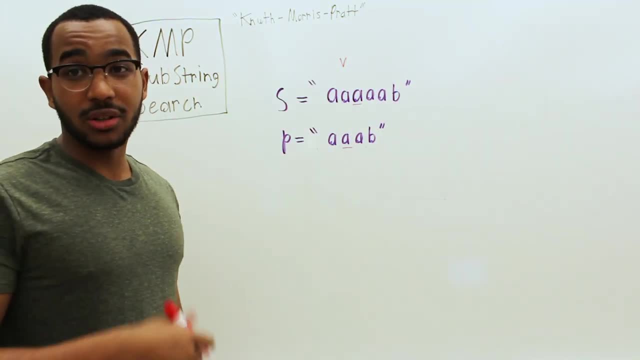 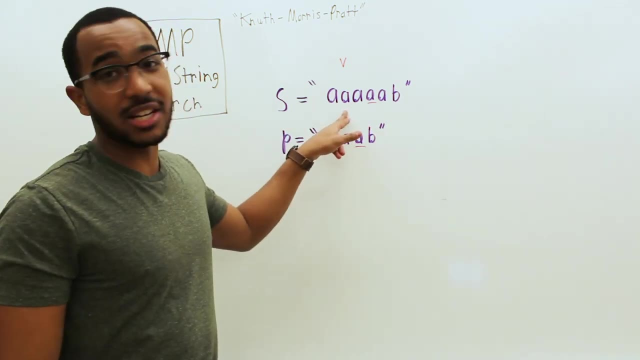 So then we go into a search. So does A and A match Yes. Continue on with the search. Do A and A match Yes. And notice we're saying if this substring started from indice 1, I should have numbered them, but if it starts from indice 1,. 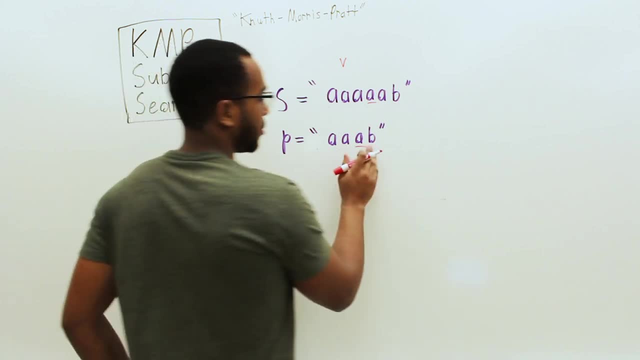 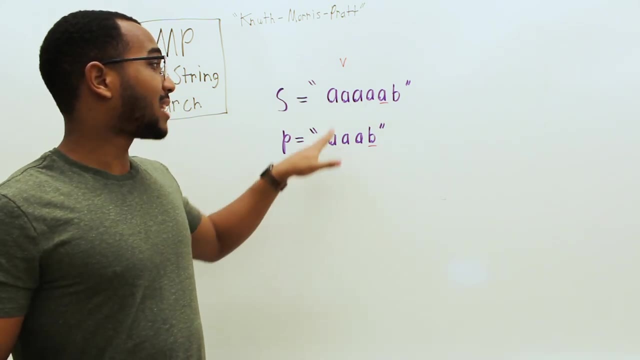 will this pattern exist? It's a match, And then, finally, we notice that these don't match, And so what we do is we revert all the progress that we made, and then we go back to the beginning and we move our search pointer. 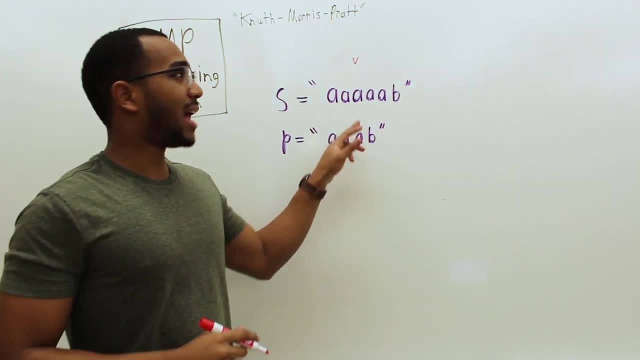 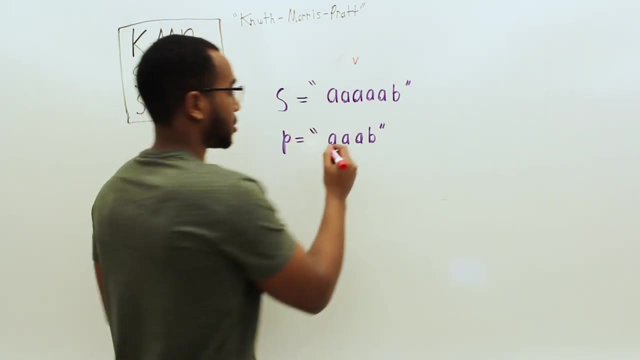 We know it cannot start here, so we move our search pointer. So now, do A and the first character of this pattern string match? Yes, they do. So go into a search. Do those match Yes, Do those match Yes. 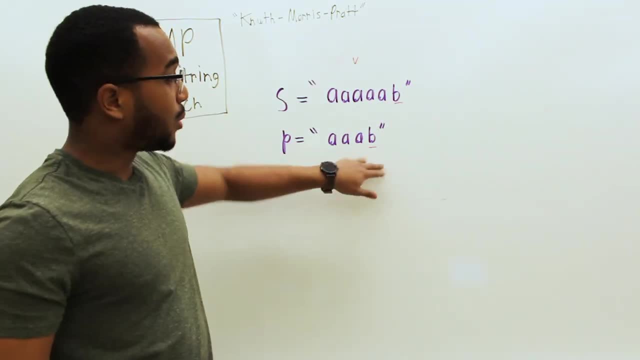 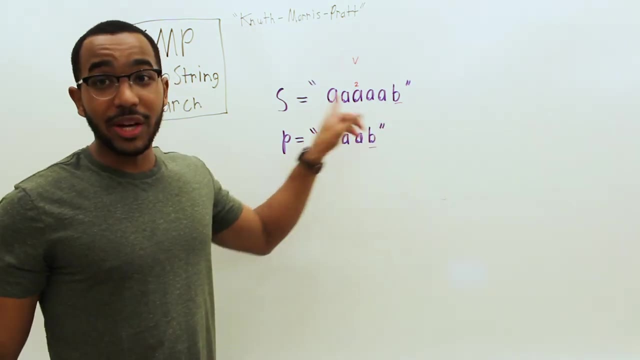 And finally, do these match? Yes, And when we go over the pattern string, then we know we've matched the whole pattern, and that means from indice 2, we know that this pattern exists in the string. So this is the naive approach. 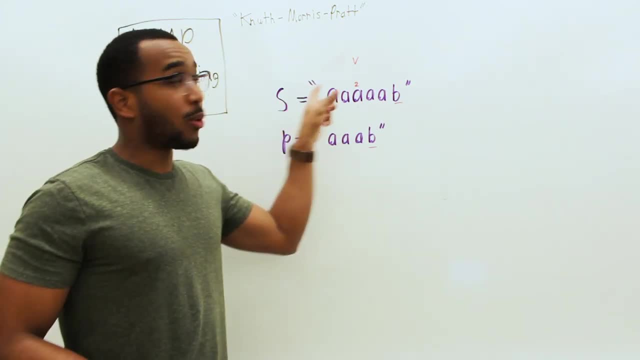 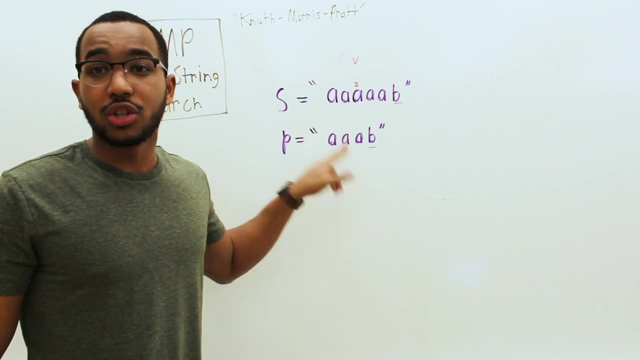 But notice, notice that for each of these, for each N, if we call, if we take the length of S, we could potentially do length of P work. So what happens is we have length of S times, length of P as our time complexity. 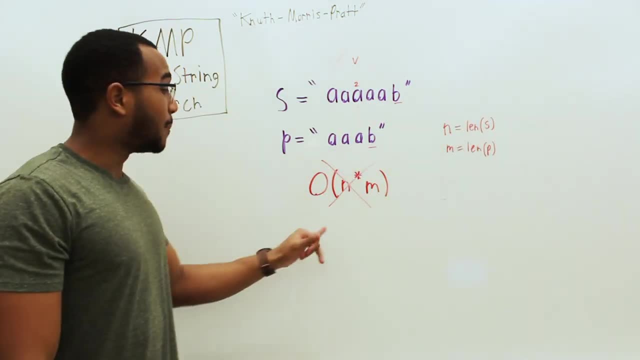 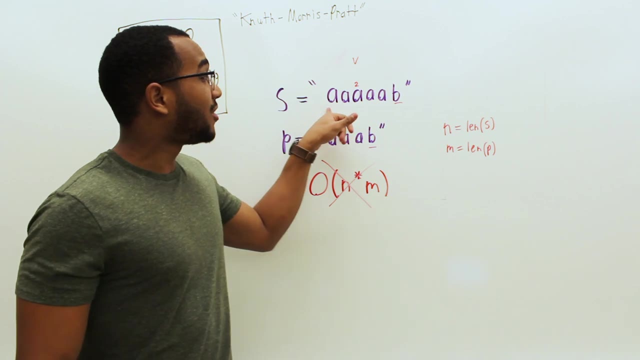 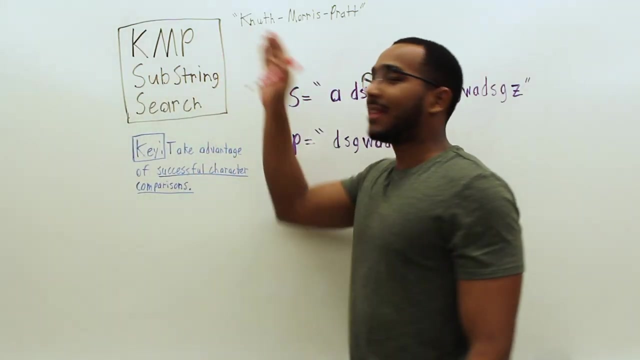 So the KMP algorithm is meant to be an improvement on an N times M complexity. This is a demonstration of the worst case, where for each of the N characters in S, we do a potential of M work Alright. so the key thing that the KMP algorithm takes advantage of: 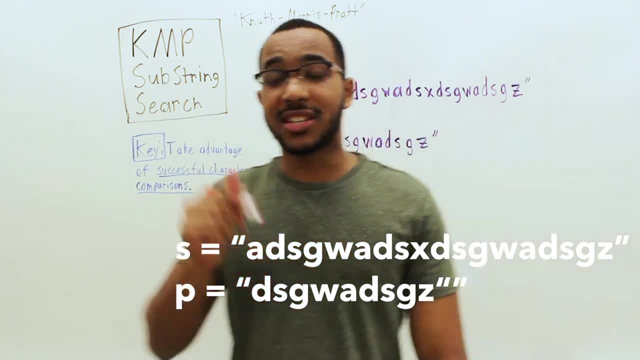 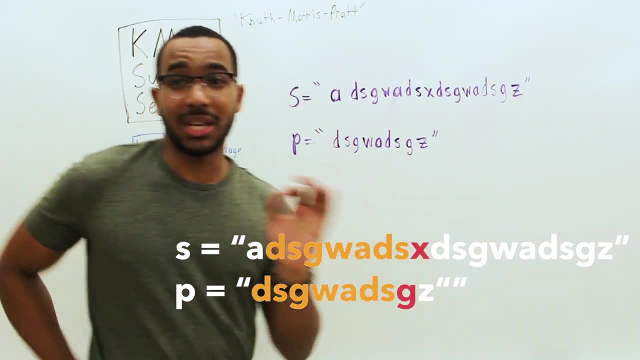 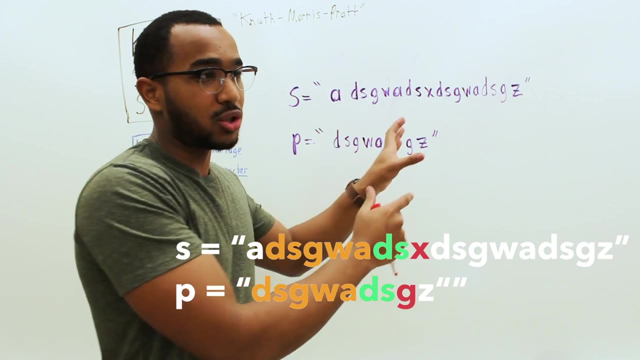 during our substring search is to take advantage of the successful comparisons that we make between S and P. We know that every character up to the character that mismatches are a match and therefore we're going to make, we're going to look for a suffix that is also a prefix. 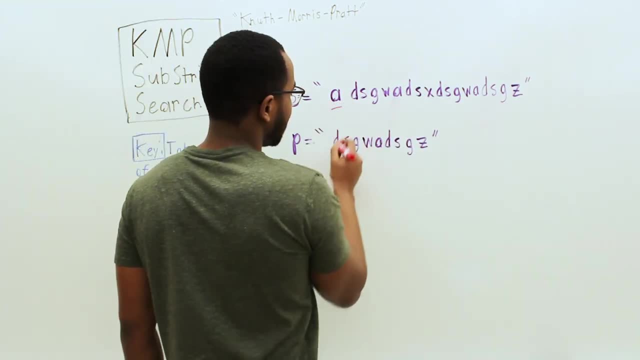 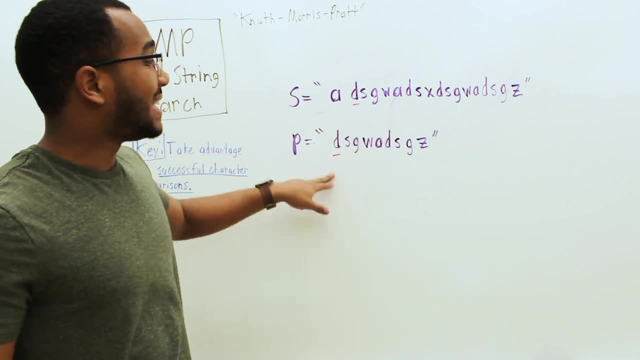 Well, we'll see in our example. So first we're going to look at A and D. So do A and D match No, So we advance forward in our string. So do D and D match Yes. 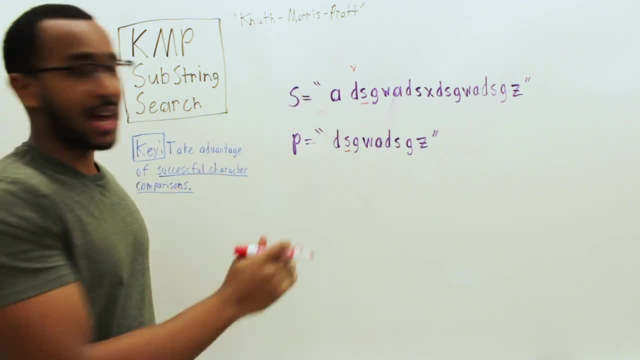 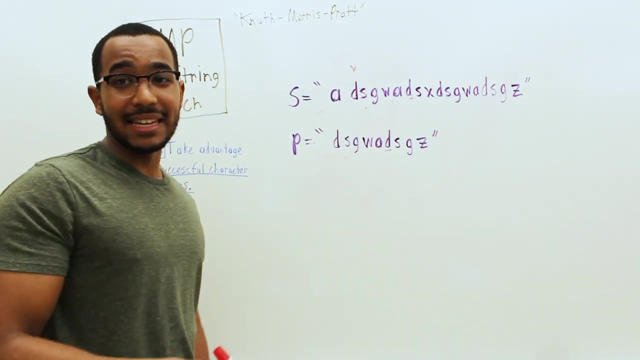 So advance forward. So do S and S match: Yes. Do G and G match: Yes. Do W and W match: Yes. Do A and A match: Yes. D and D match. Do S and S match: Yes. 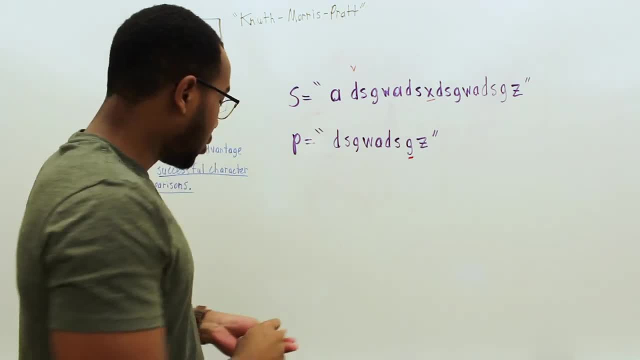 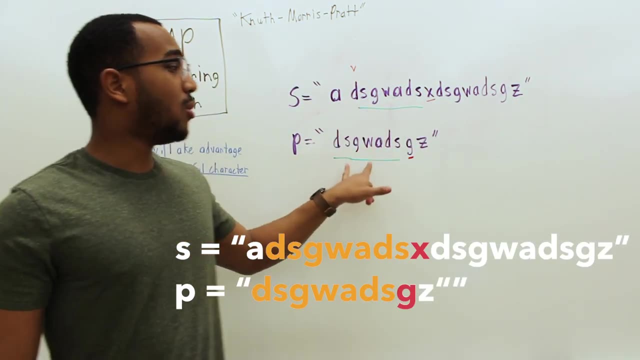 Do X and G match? They do not match, But notice something. So what we've done so far is what I just underlined in green, is what we have matched so far. We know that this, this substring, this part of the pattern string. 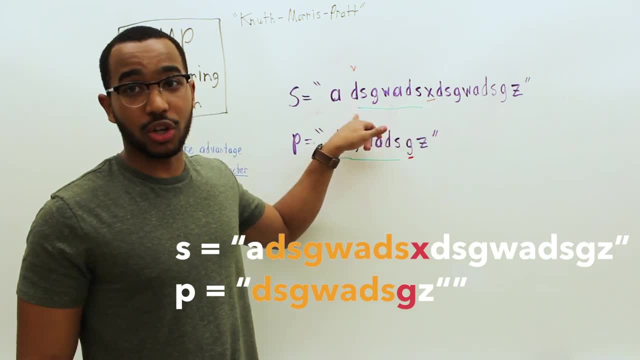 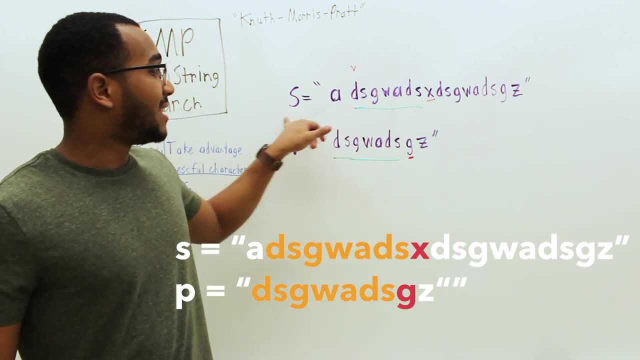 exists in our string starting from this search index. So what the KMP algorithm does is we want to prevent ourselves from going backwards in this, in this string, and reverting our progress in matching the pattern. So we know that these match. 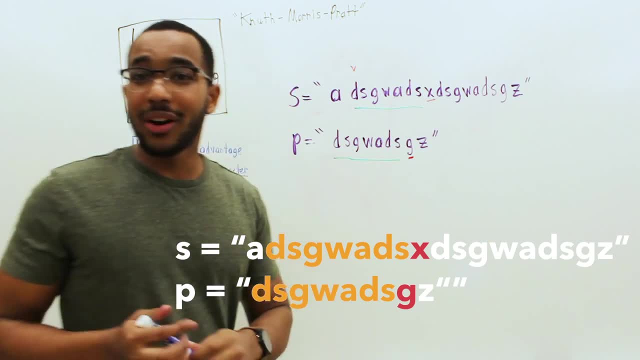 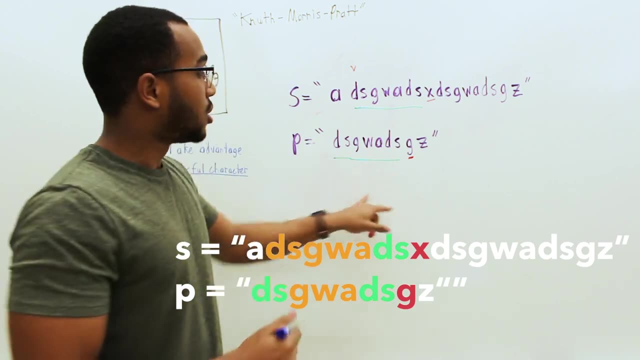 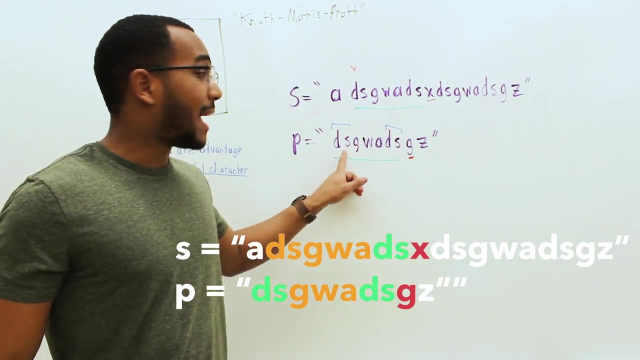 So what we need to look for is we look for a suffix that is also a prefix in this character, before the mismatch. So what we see is that D-S, D-S, D-S. this suffix is also a prefix. What do we know? 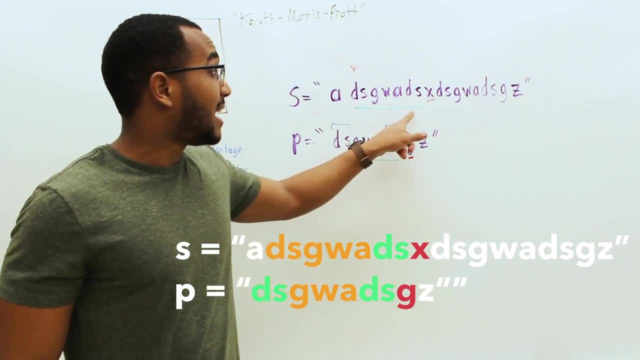 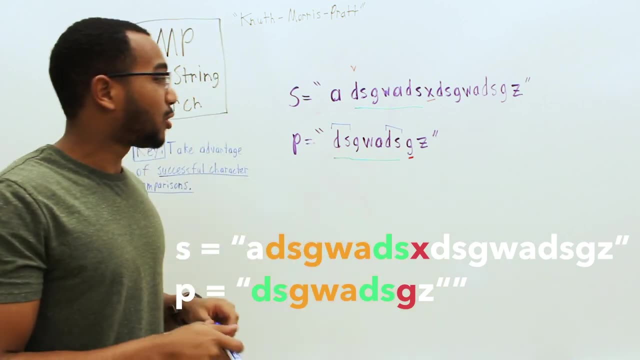 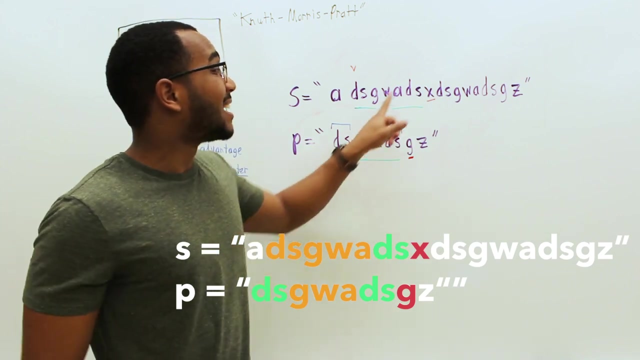 We know that D-S exists in this string. from here, We know that D-S exists before our mismatch. So what the algorithm does is it says, hey, how far back do I need to go backwards in my pattern so that I can not revert my progress? 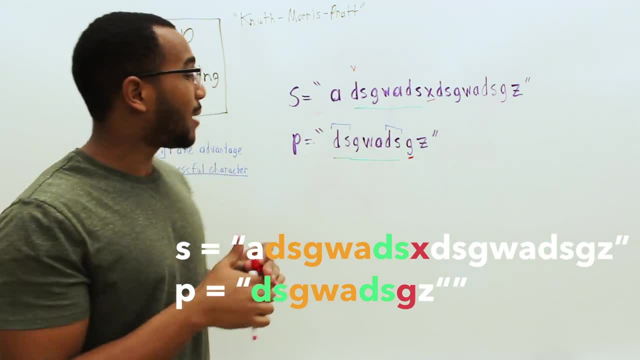 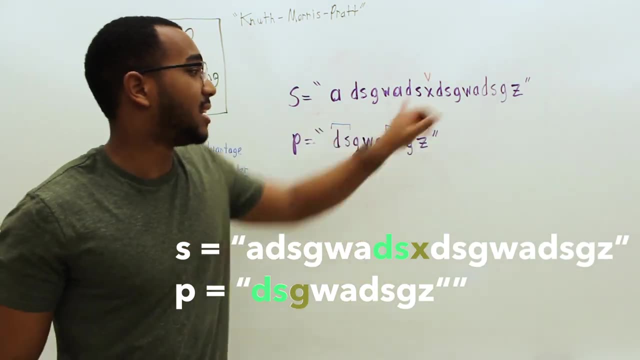 in the string that I'm matching to, The key place that we jump back to is we jump back to this G. So we mismatched X and G. G and X did not match And we know that everything before it did match. 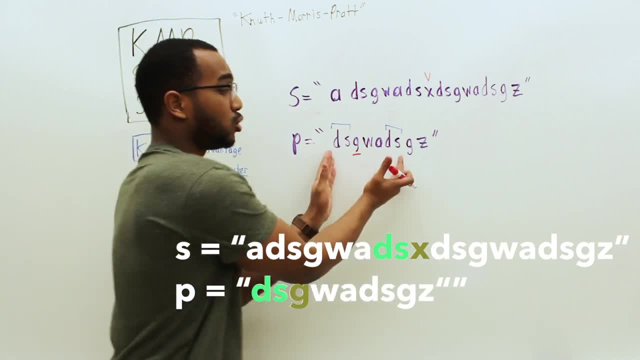 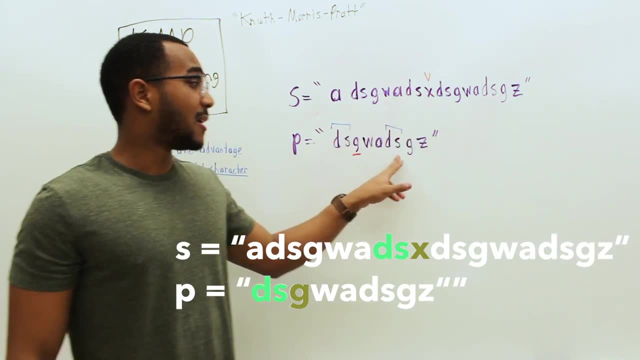 So if we can find a suffix to this substring that is also a prefix, then we are able to continue our search from where the mismatch is, because we know these two match in sequence. So if we can find a beginning of the string, 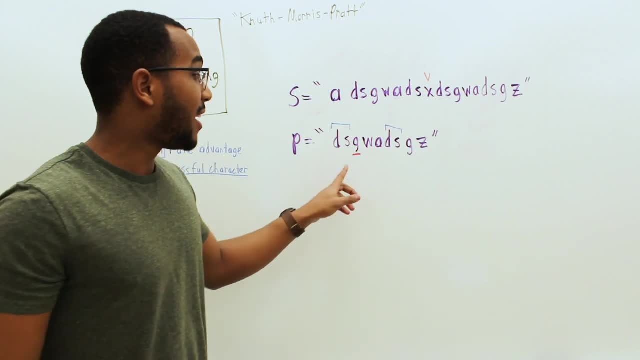 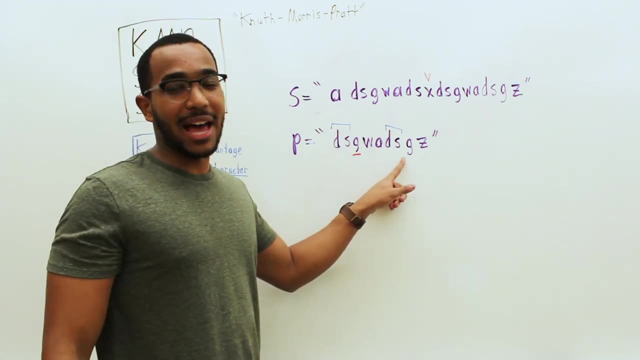 that also matches in the same sequence. then we can just continue our search from after. what we know won't match. So we know, okay, we know D-S will match, and then we have a mismatch. So then we know if this is a suffix. 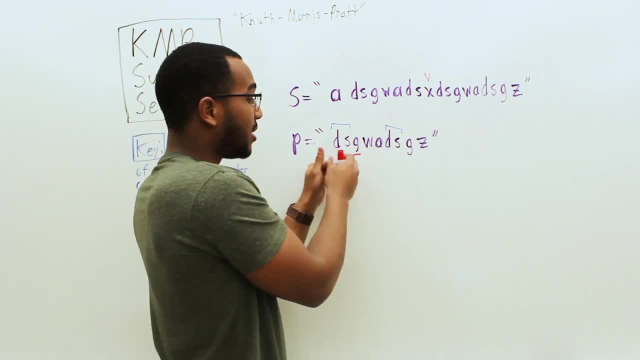 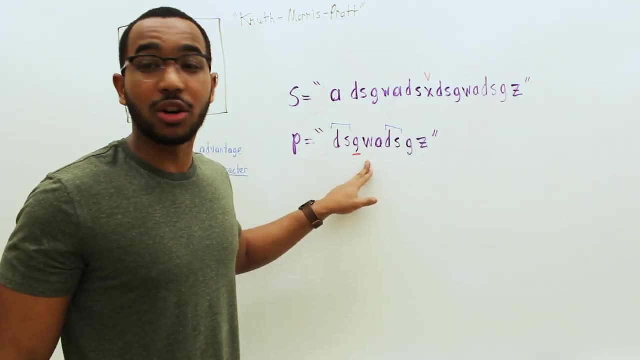 to the substring before our mismatch. then we know that our prefix is going to also exist in this string. and then we know we need to continue our search: one, two, three indices forward, from the D and the S And, as you can see, 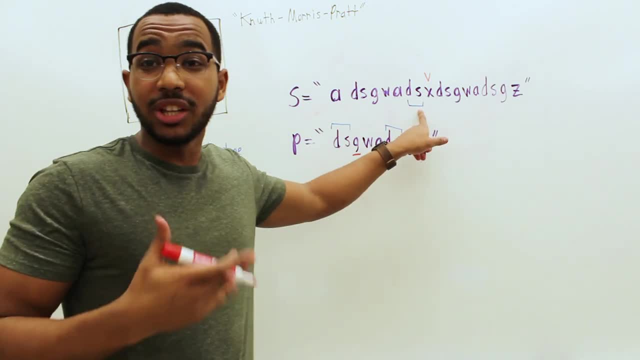 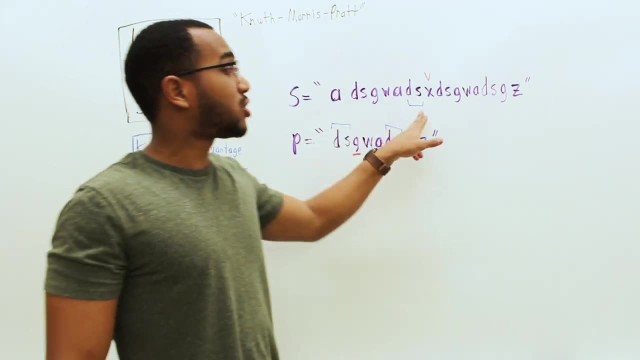 D-S does exist in the string, because we literally just matched that. So this prevents us from going backwards in our search string. It allows us to continue our search from the D and the S, which is a prefix here, and it allows us to just continue from the G. 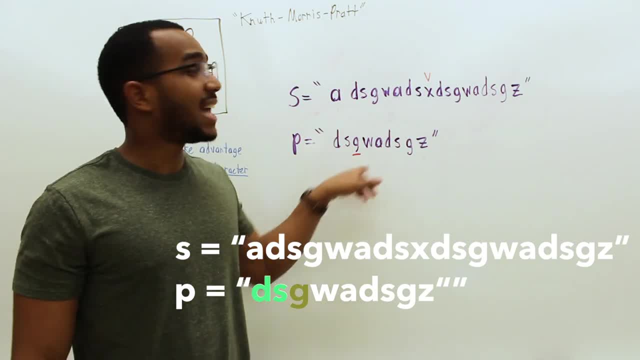 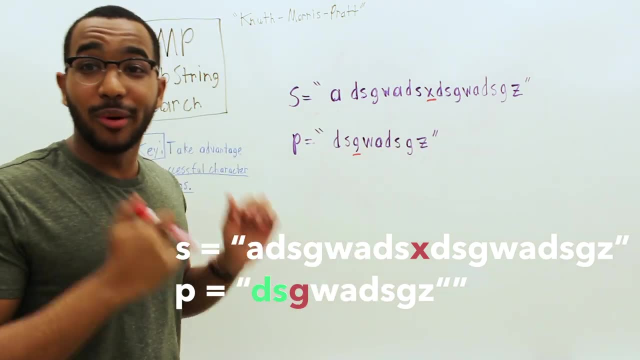 So we continue from the G. So now we're going to compare G and X, Now we're going to compare G and X and we have a mismatch. So again, what we do is we try to prevent going backwards in progress. 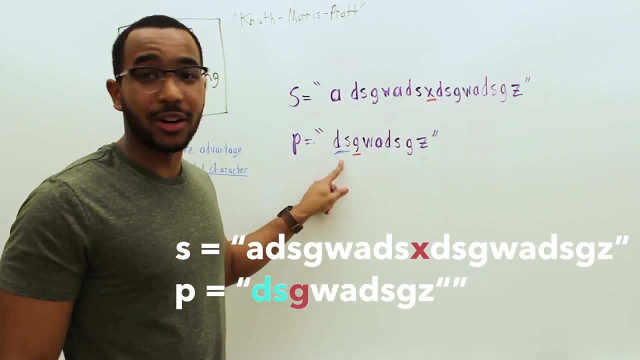 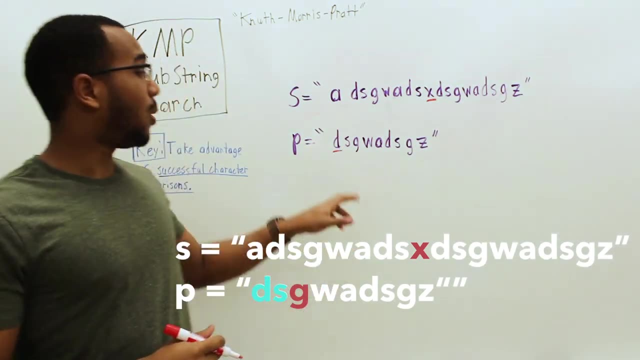 So we look here, We look at the substring of D, We look at the substring of the pattern D-S. Is there a suffix? that is also a prefix, And what we see is no, there is not. And so what we do is: 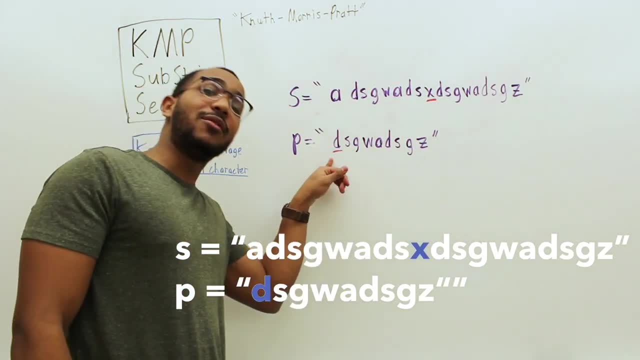 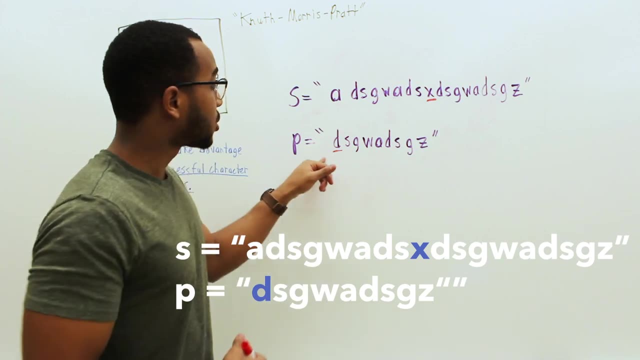 we have to revert all of our progress. We have to go all the way back to the beginning of our pattern string, because we were not able to find a suffix. that was a prefix that could save us from going backwards in our work. So we compare the D and the X. 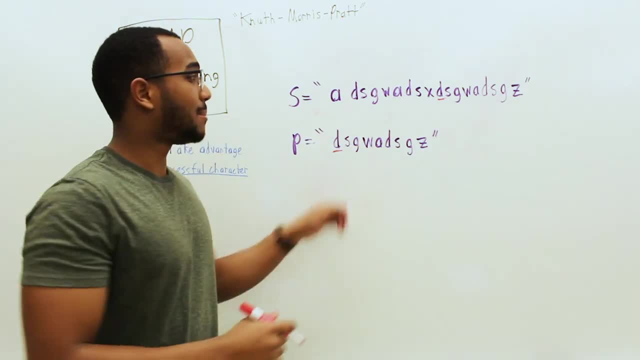 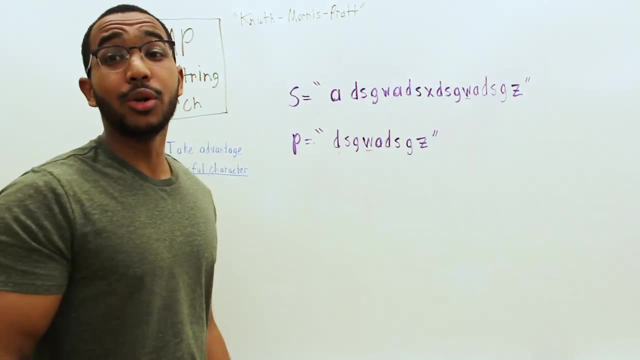 They don't match. So we just continue doing our checks so that we find D and D match, And then now we're going to go into our matching: S and S match, G and G also match. W and W match. 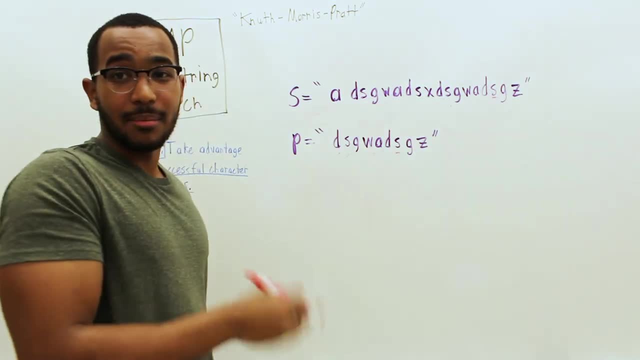 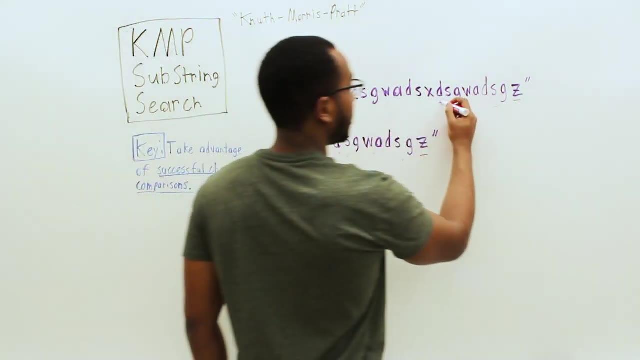 A and A match, D and D match, S and S match, G and Z match And then finally Z and Z match, And we found a pattern in our string and our answer is right there. So the key is: every time we find a mismatch, 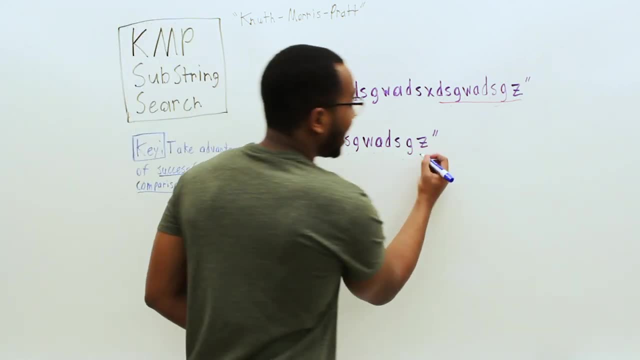 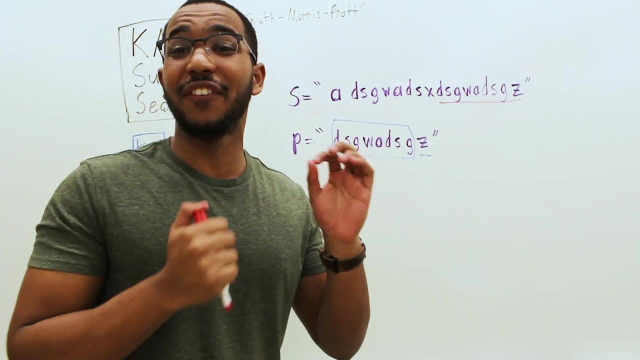 we're going to ask ourselves, We're going to say behind the mismatch, So say the mismatch is at Z, Behind the mismatch, Behind the mismatch, Can I find a suffix? that is also a prefix. So, since we know that we matched D S, G, 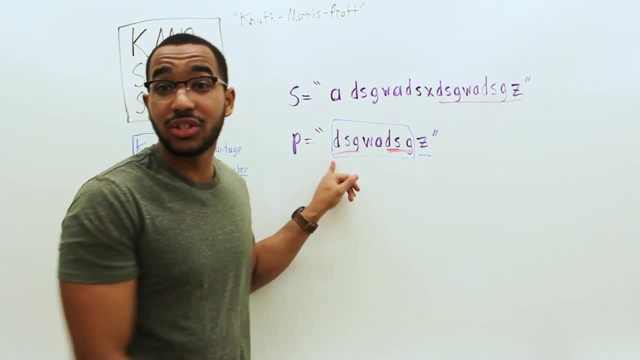 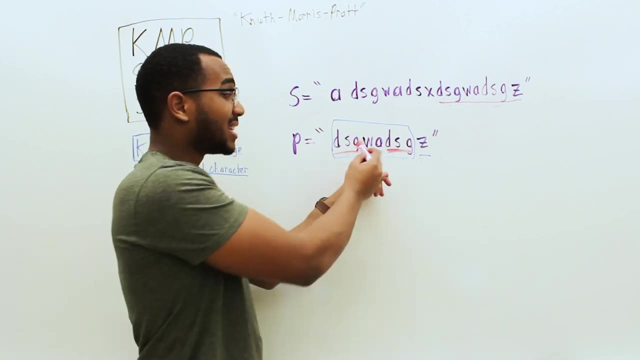 and then we found a mismatch at Z. we know that we can just go back to the beginning of the string. We know we matched D, S, G, We know those matched. And then we can just hop, We can say, let me start matching at W again. 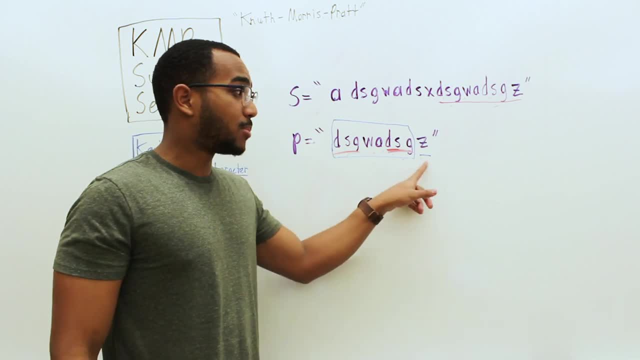 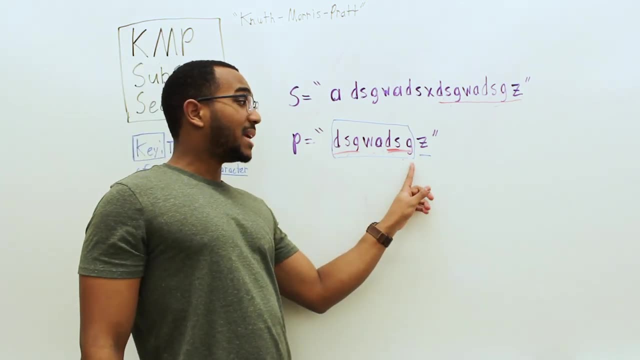 So it's saving us these checks because we know all of these match up to the mismatch. So it would make logical sense that to prevent backwards motion we want to find the characters behind the mismatch that are also at the beginning of the pattern string. 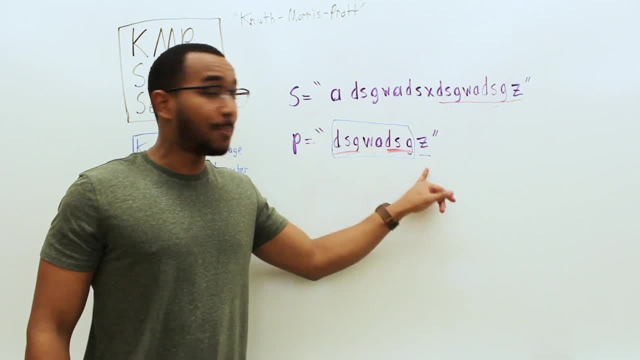 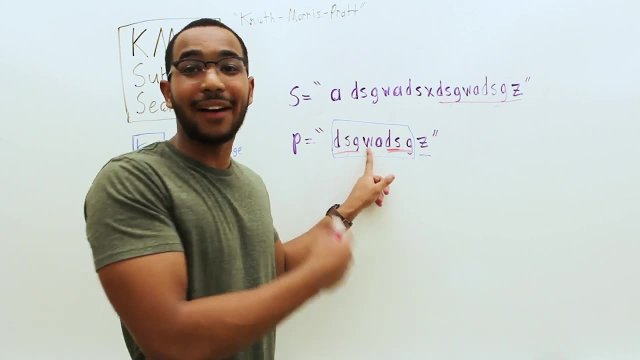 because we can skip these checks. We've already matched these up to the mismatch. We can skip these checks at the beginning of the pattern and we can just continue on to where it does not match, which is after the prefix. that is also a suffix. 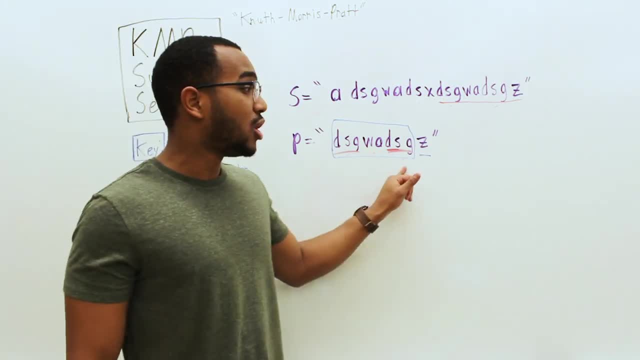 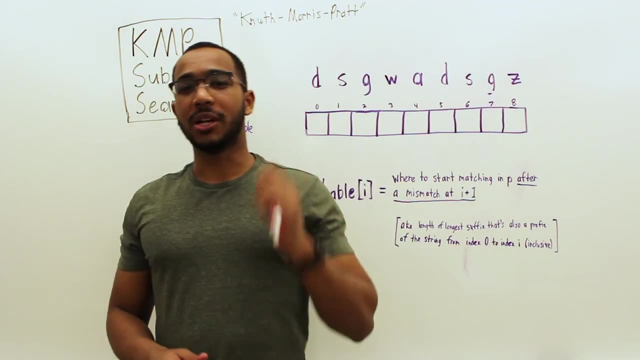 This is why prefix and suffixes matter. It allows us to not repeat work in the pattern, so we don't have to revert progress in the string. So what we do is we build a prefix suffix table, So each of these boxes represents a substring. 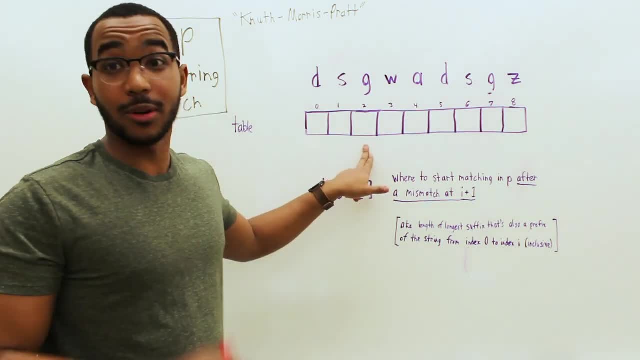 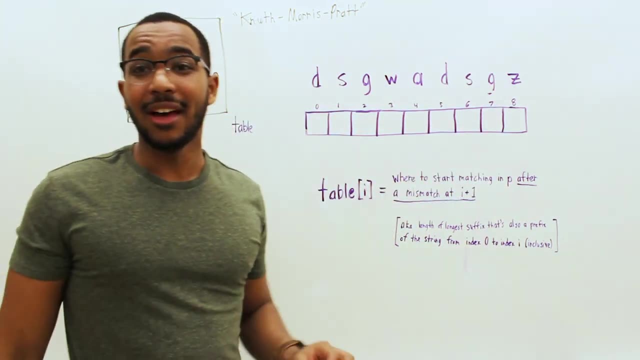 So if we see box 2, it represents the substring from 0 to 2 inclusive. So this substring, which is D, S and G, So each of these boxes, tells us the length of the longest suffix. that is also a prefix. 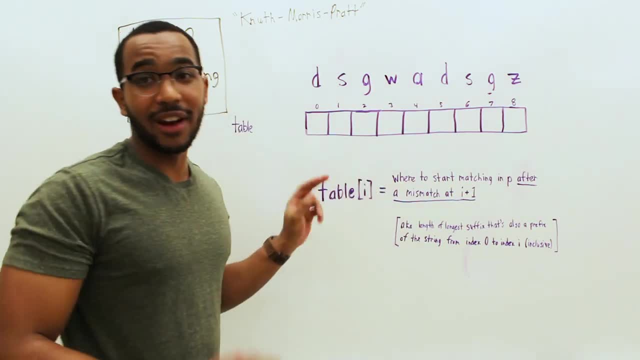 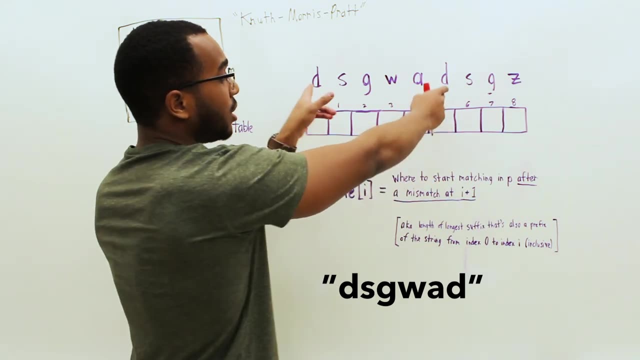 from here to here. here to here. Whatever that cell is, it indicates the substring we're taking. If we were just looking at this, the longest suffix, that is a prefix up to 5, we know it's going to be 1. 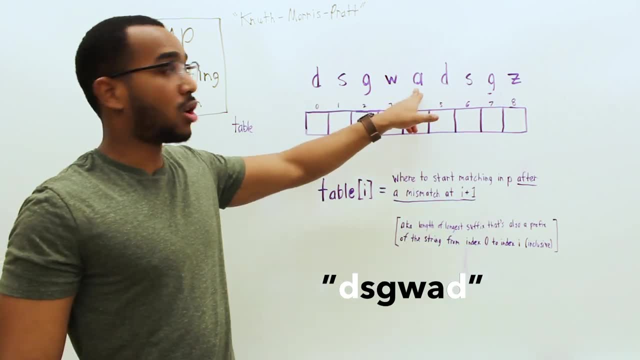 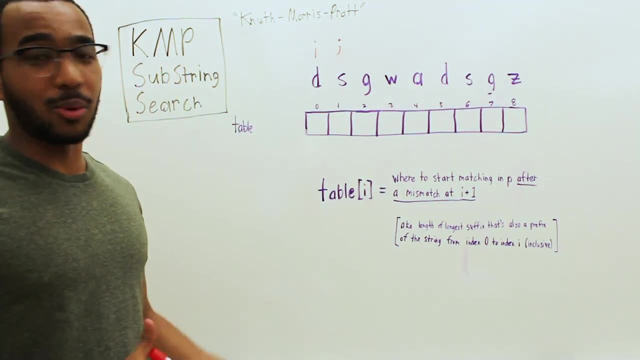 because the suffix D is also a prefix, which is D. But we can't go longer. AD is not a match as a prefix. What we're going to do is fill out this table, So we're going to have two iteration pointers, I and J. 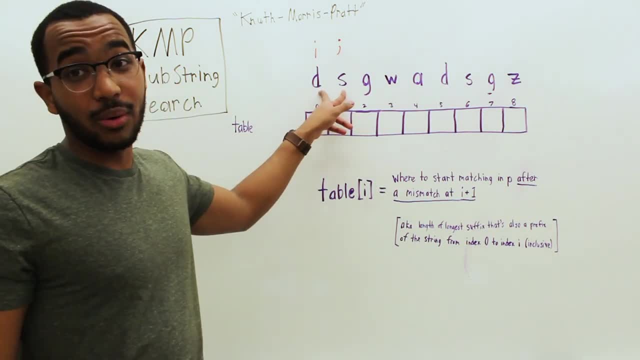 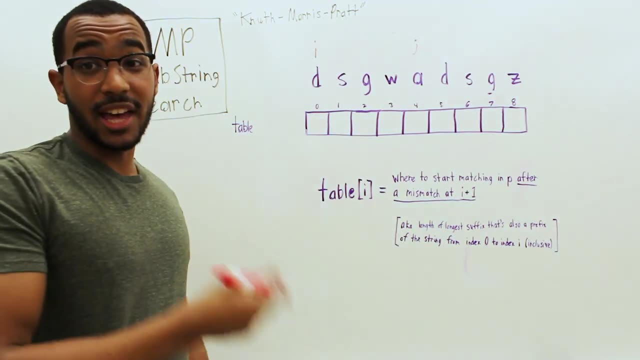 So we're going to compare I and J. Are they equivalent? If they're not equivalent, then advance J Not equivalent, advance J. These are not equivalent. so advance J, Advance J again. So every time that we find that these are not a match, 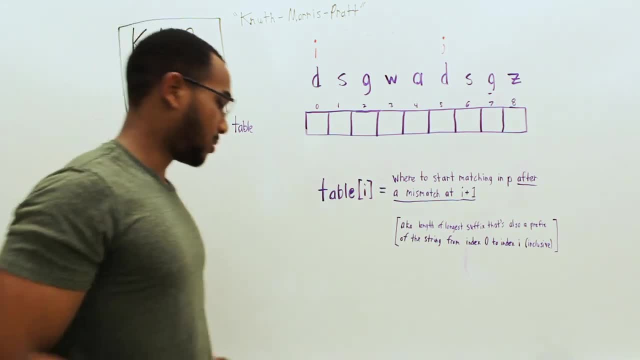 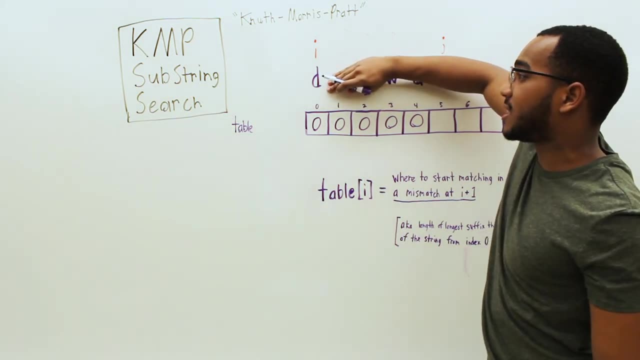 initially after no match, we just put a 0. So what this is saying is for each of the substrings. So for the substring of just D, the longest suffix- that is also a prefix, is length 0.. Length 0 for D and S. 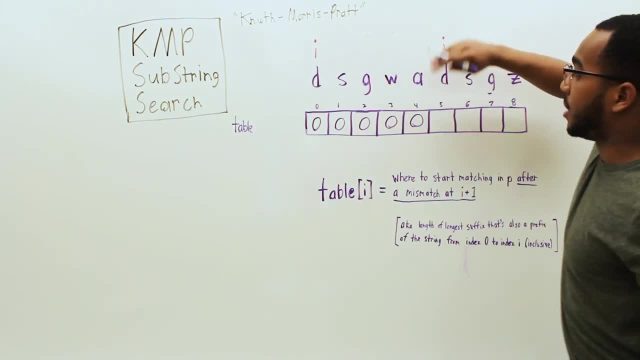 Length 0 for D S G. Length 0 for D S G W. Length 0 for D S G W A. So that's what these zeros mean. It means that our longest prefix and suffix does not exist. 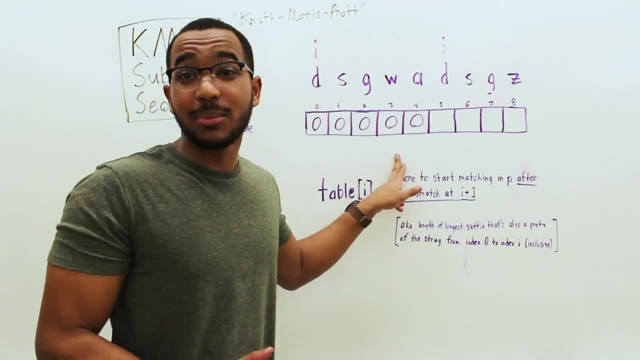 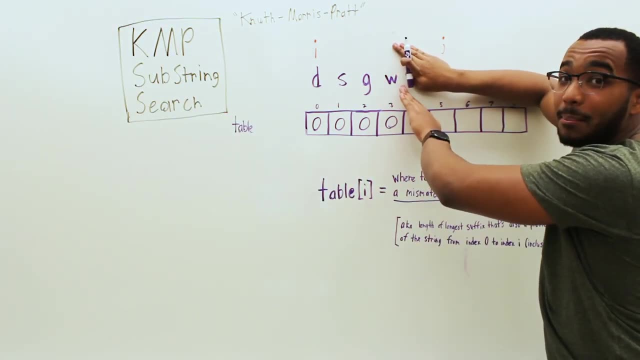 Each of these is telling us if we find a mismatch at I plus 1,. if I find a mismatch here, give me information about the prefix suffix data for I minus 1.. The substring behind me, Which is literally what we were doing before: 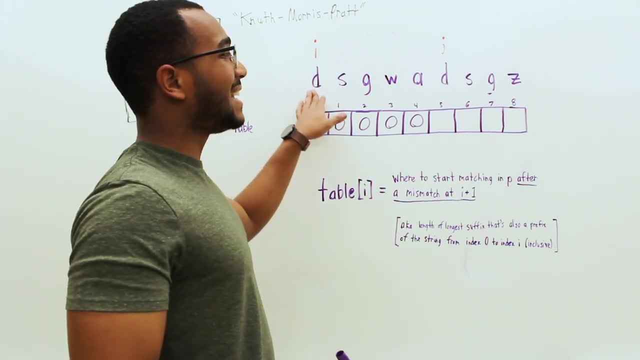 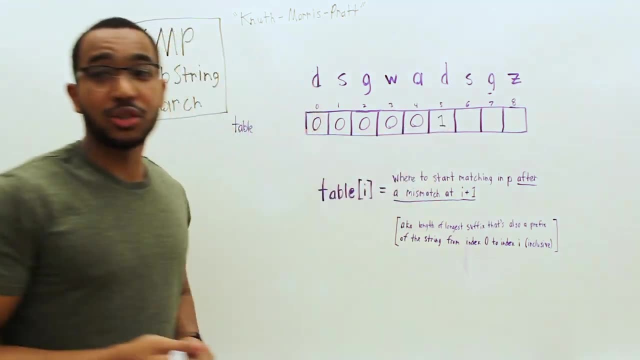 That's what this table is about. So anyway, continuing with the iteration, we see D and D match, So we do I, which is 0, plus 1, into this cell, And then what we do is we advance I and J by 1.. 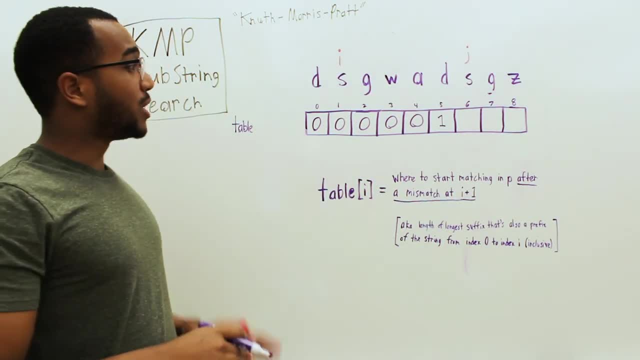 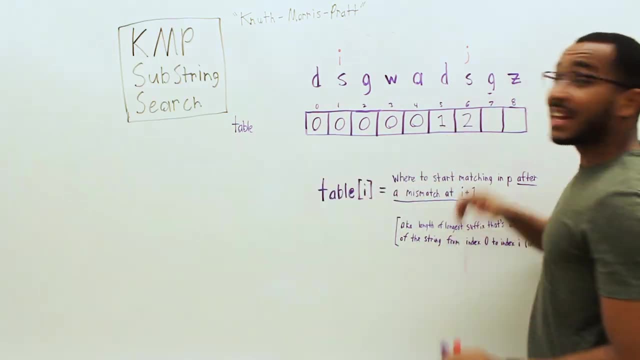 And now we see that I and J match. So we do I plus 1 into where J is. So we do 1 plus 1, which becomes 2.. And again this tells us. so what that 2 in that cell tells us. 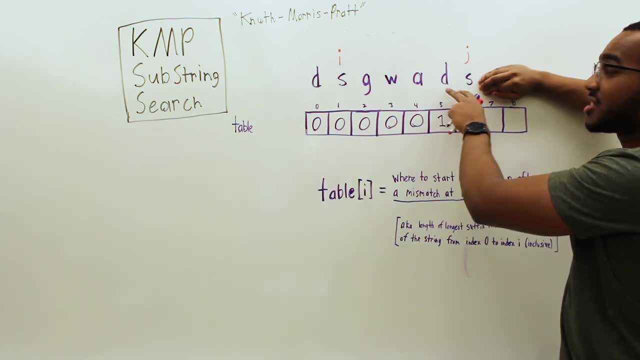 the D S, G, W, A, D S. the longest suffix that is also a prefix is length 2.. We can see that D S, D S. So if we have a mismatch here plus 1,, 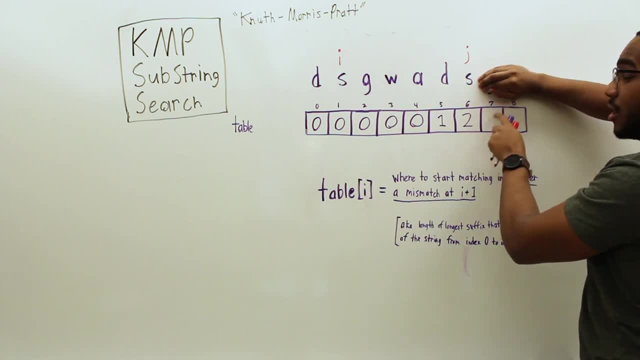 if we have a mismatch here? if we have a mismatch here, we know we're going to have to look at this substring. And when we look at this substring, we know we've already matched D S up to the mismatch, So we can just go D S. 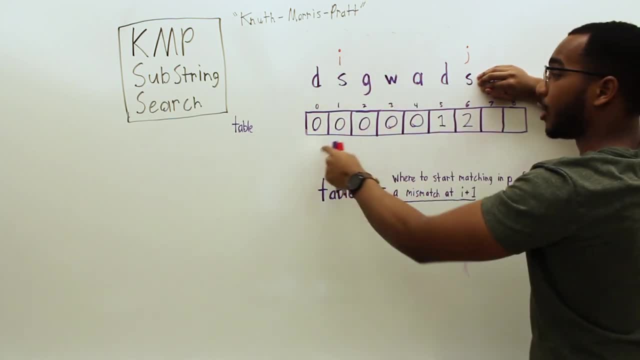 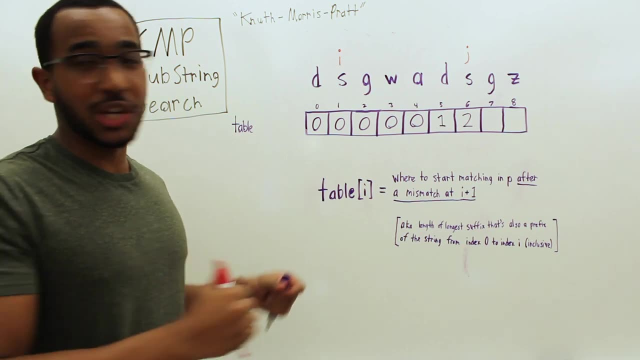 and then we can just match here G which 2, 0, 1, 2.. This tells us the index to continue our matching gap. So that's what this is all about. That's a match. So now we need to increment I and J. 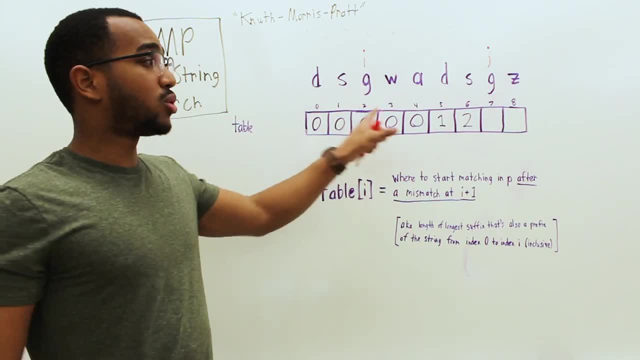 So now G and G match. So we're going to do I plus 1.. 2 plus 1 is 3.. So 2 plus 1 is 3.. And what does 3 mean? Let's do this again. 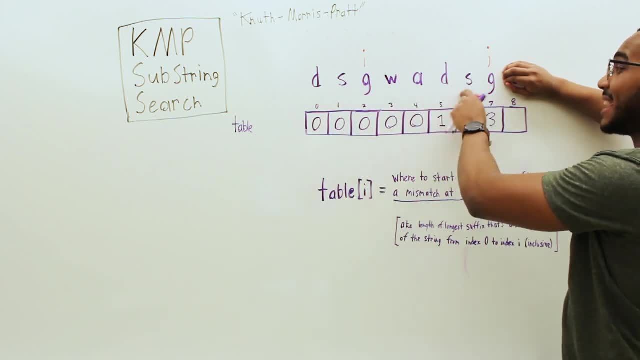 If we have the substring D S G, W A D S G, if I find a mismatch after this substring, if I find a mismatch over here, whatever that is, I need to know about this substring. This cell gives me information about this string. 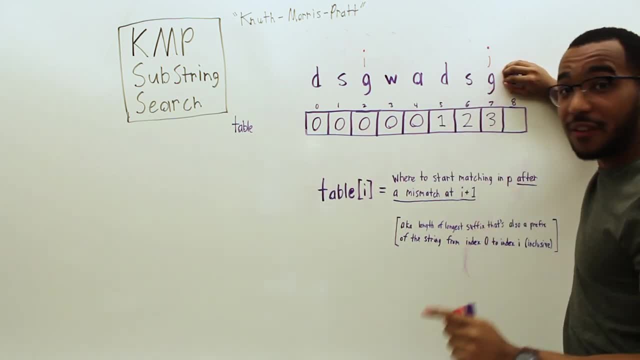 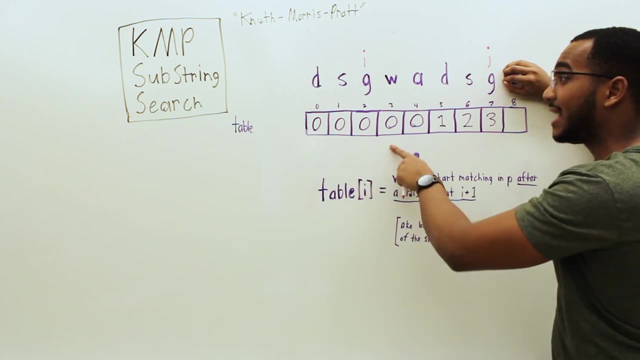 It tells me the suffix, the longest suffix, D S G. That is also a prefix. D S G is of length 3.. 0,, 1,, 2,, 3.. So I continue my iteration. 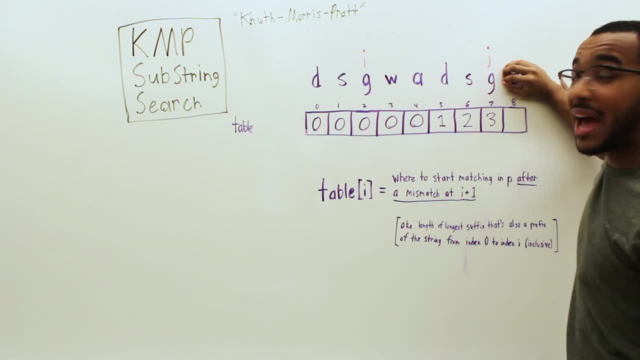 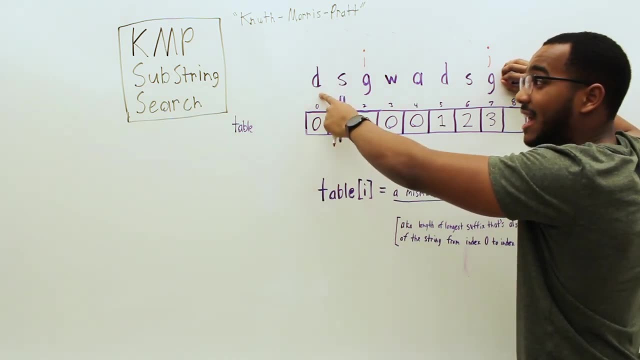 I continue my matching from W. Why do I do that? I already matched D S G. If I have a mismatch here, I know I can save that progress. I can say D S G is at the end, It's at the beginning. 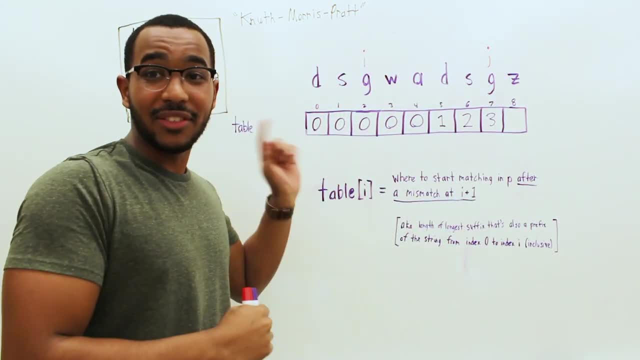 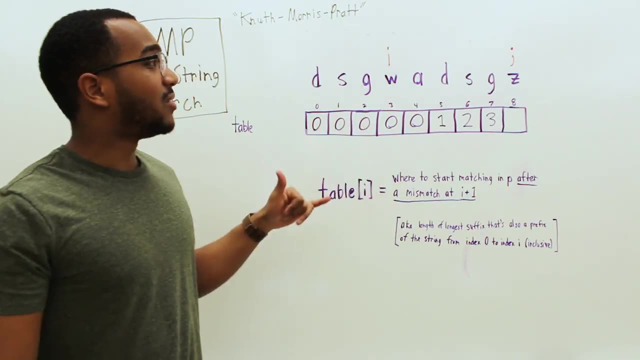 I can save that progress. This table is all about how do we save that progress. So now we matched I. We need to advance I and J. So now we have a mismatch And this is kind of weird. but what we do here is we look at I. 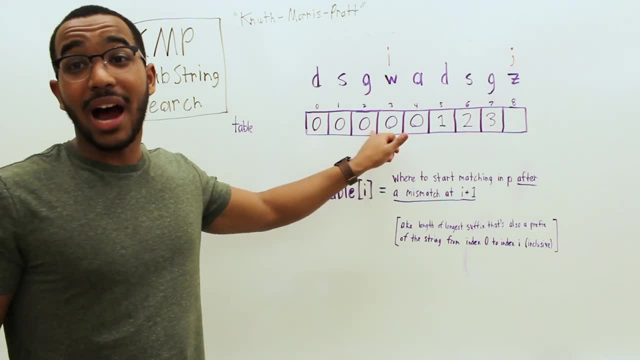 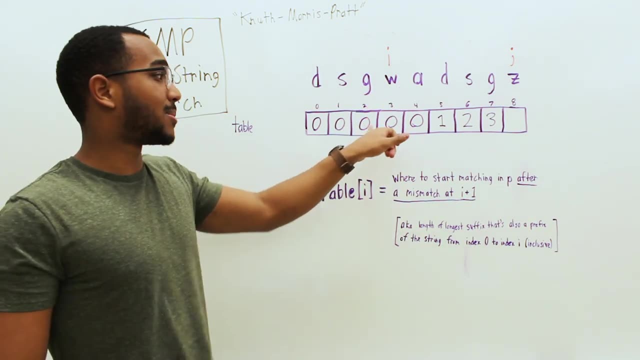 and we look at the value at I minus 1 and that is what I becomes. I becomes the value at I minus 1.. So it doesn't become the 2.. It doesn't become the index at I minus 1.. It becomes the value. 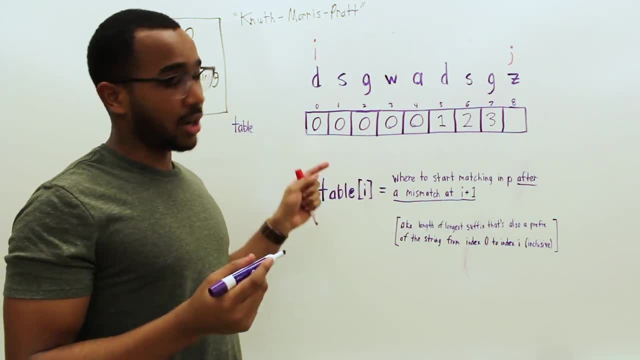 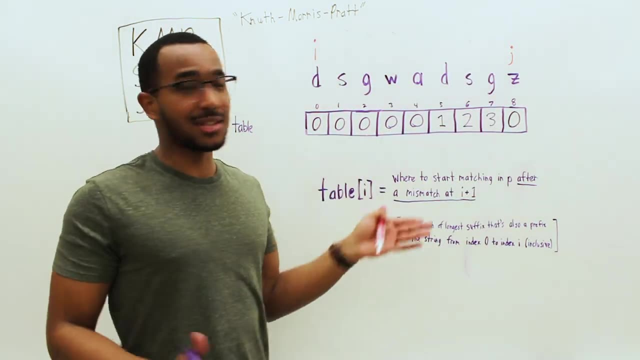 So I becomes 0 here. So D and Z are not a match here. So what we're going to do is put 0.. So if you look at the whole string, the longest suffix- that is also a prefix- does not exist. 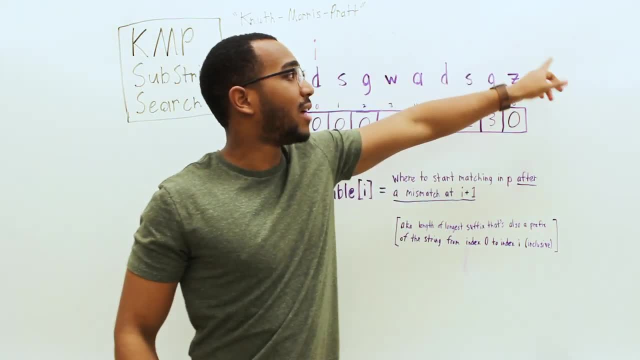 So it's just 0.. If we try to increment J, we're going to run over the array. It's going to go over here. So this is our prefix suffix table. And now what we need to do is we can walk through an example. 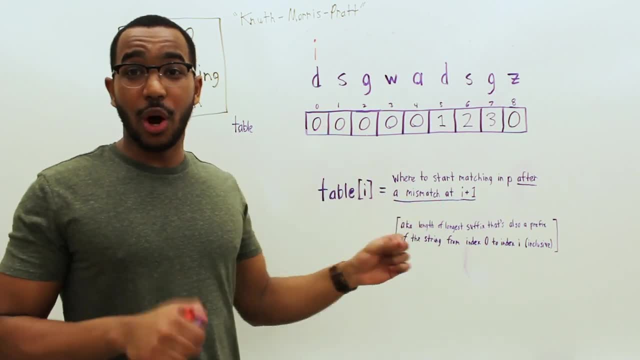 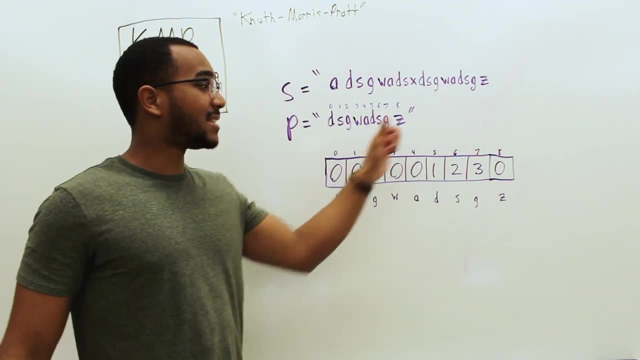 and look at this. How is this table going to help us know where to jump back when we have a mismatch? So let's see how this helps us. Alright, So now let's go back through the matching. I've numbered the indices in our pattern. 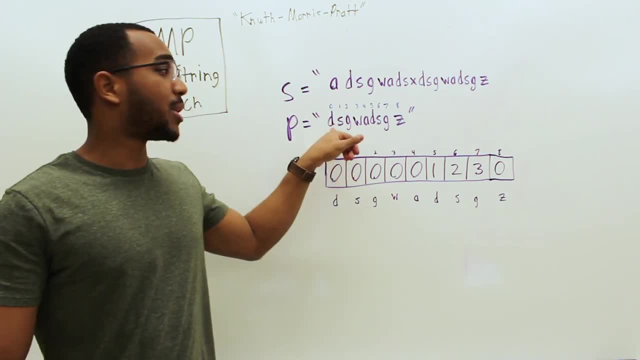 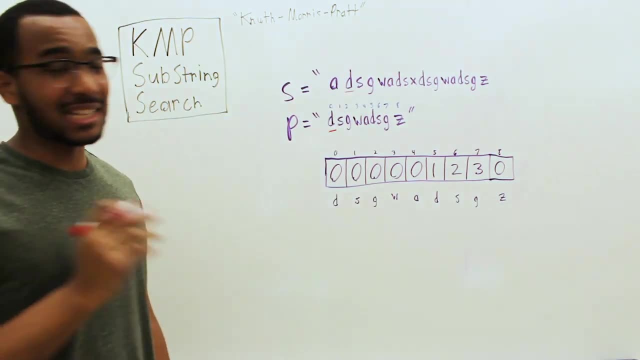 This is going to show us how our table influences, how we go back in our pattern by indices. So let's do our comparisons again. We compare A to D- No match. We compare D to D: That's a match, S is a match. 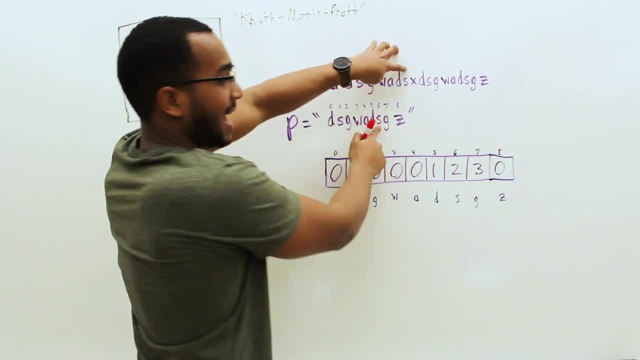 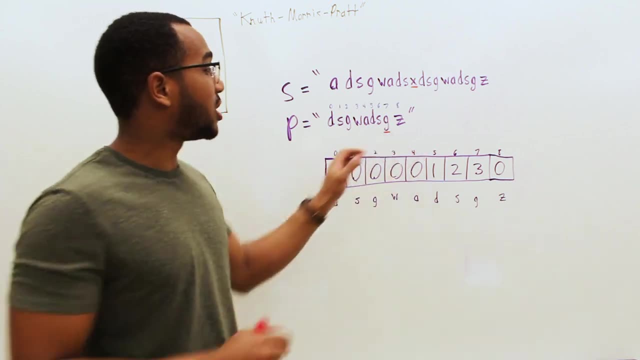 G is a match, W is a match, A is a match, D is a match, S is a match And then G, So we have a mismatch at indices 7.. So what we need is: we need information. We've matched. 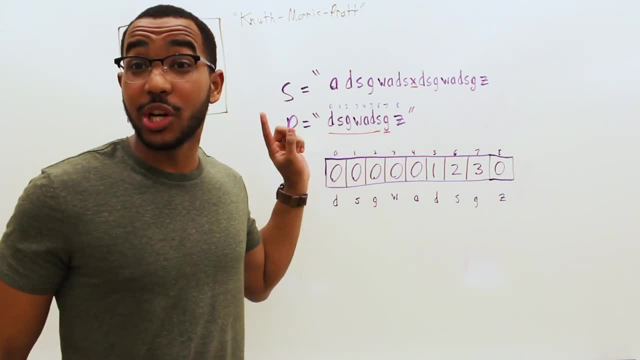 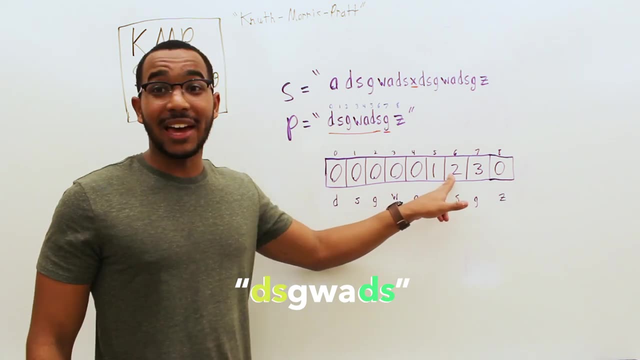 What we've matched is we've matched the substring from 0 to 6.. And remember, we have information on that. We now understand that the longest prefix, that is also a suffix, the longest suffix, that is also a prefix that goes from index 0 to 6,. 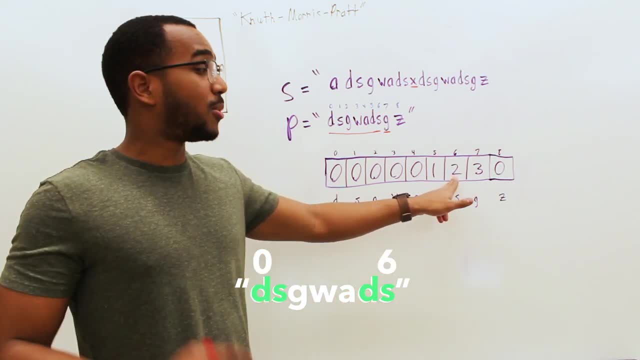 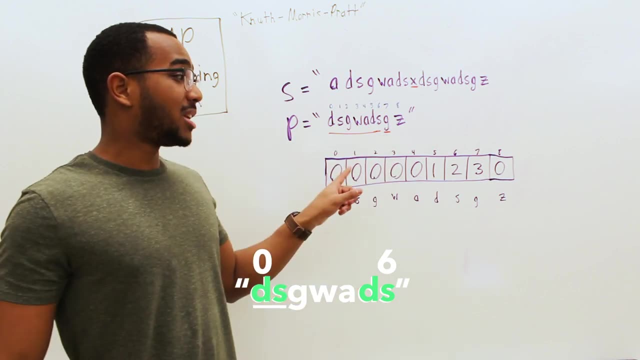 the substring of the pattern we know. the longest suffix, that is also a prefix, is 2.. The length of it is 2.. And notice, it is 2. DS, DS. So right before our mismatch, our mismatch happened at indices 7. 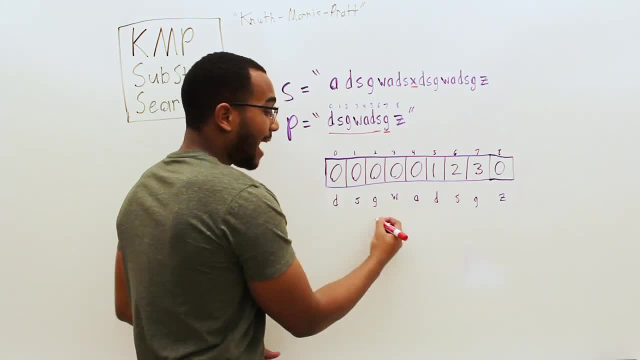 and we know we need information on this. So we know, now we can start our search. We can start our search from 0,, 1,, 2.. We can start our search from 2, because the length of this is 2.. 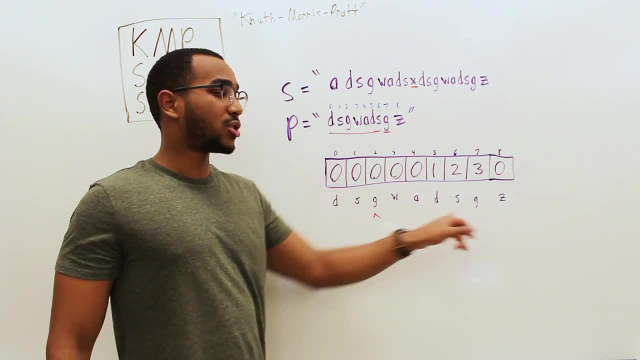 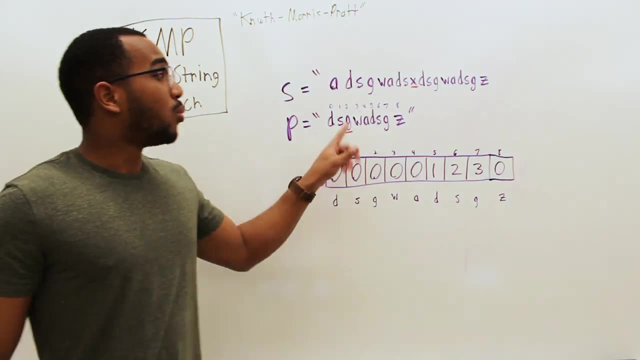 We know this: matches: We know DS G Mismatch. We know that matches Come back to the start Match match Mismatch. So we know we need to start from here, Start from the G. So now we've prevented backwards progress. 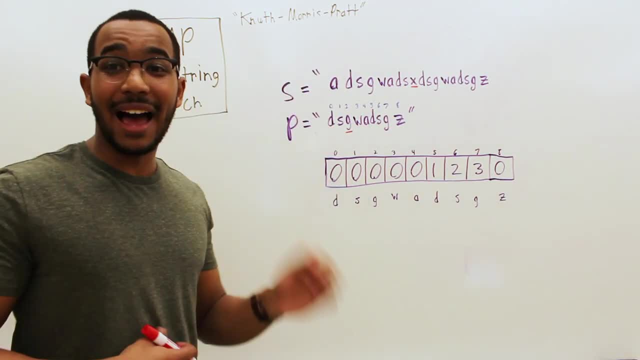 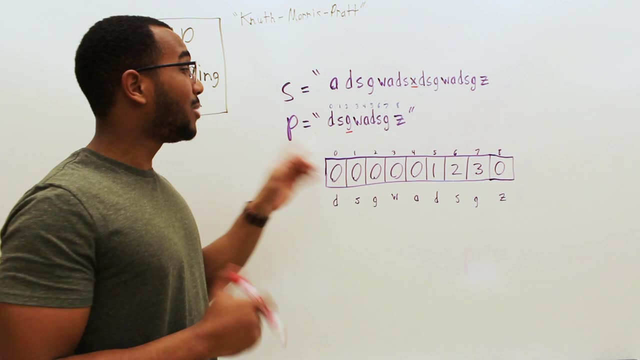 in our string S, our search string, And this is what makes this allow us to run in linear time with respect to the length of S. Now we compare G and X. It's a mismatch. So now what we need to know is: 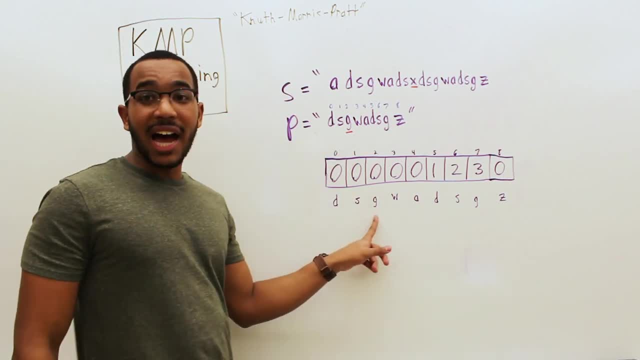 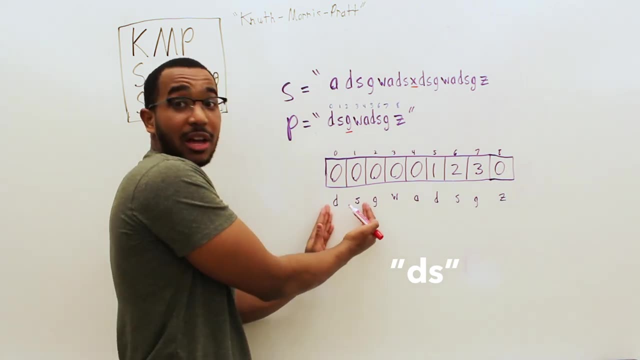 for my substring where my mismatch happens here. I need to know about the substring from 0 to 1.. I need to know what happened right before my mismatch. What about this substring? What is the longest prefix that is also a suffix? What is the longest suffix that is also a prefix? 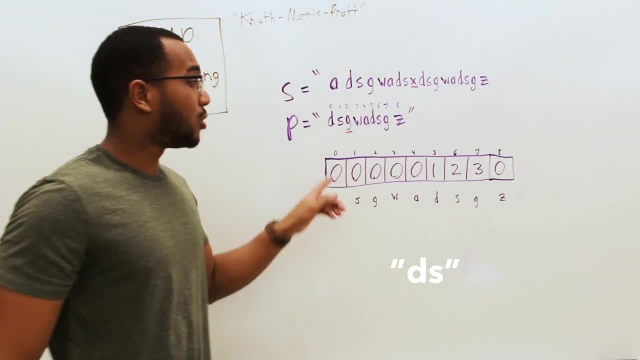 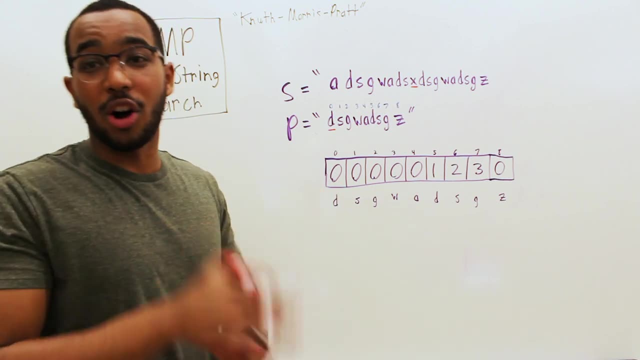 that goes from index 0 to 1? 0.. So now we know we need to come back all the way to the start, to D. We were not able to save ourselves work. Now we need to come all the way to the start. 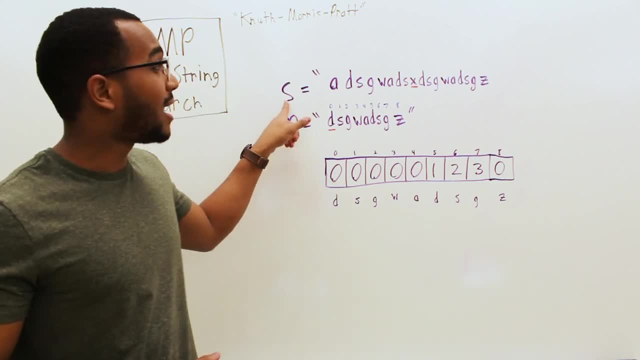 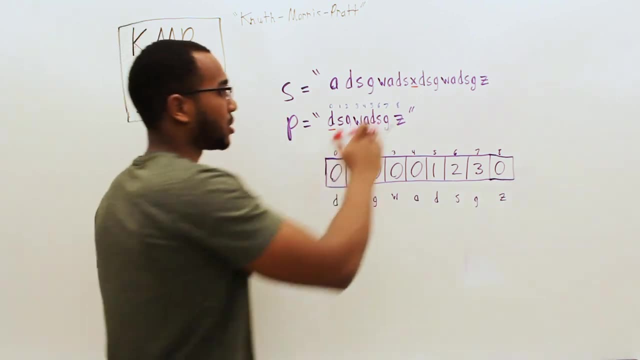 And notice we're staying linear with respect to S. We're not redoing work, We're not going all the way back. This is saving us progress. We compare D to X. It is a mismatch. So we compare D to D. 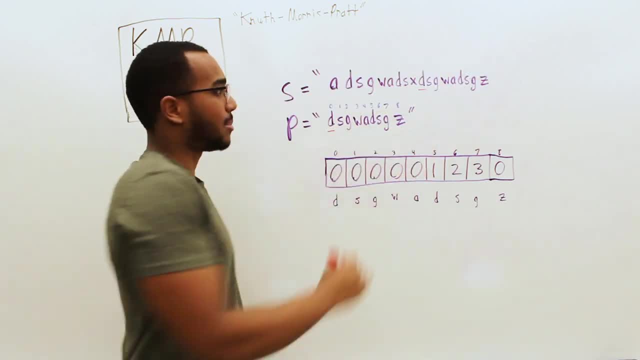 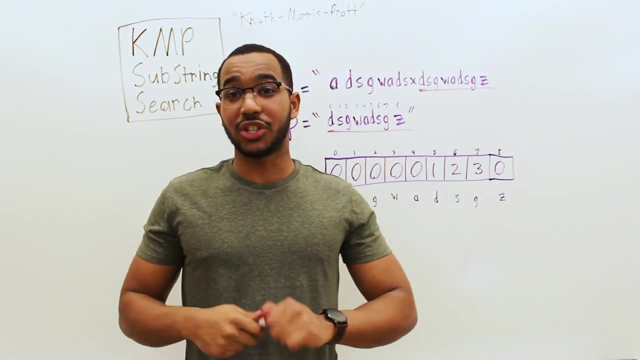 S to S, G, W, A, D, S, G Z. That's a match. So this is our substring. This is what K and P substring search is all about. This is not the only linear time substring search algorithm. 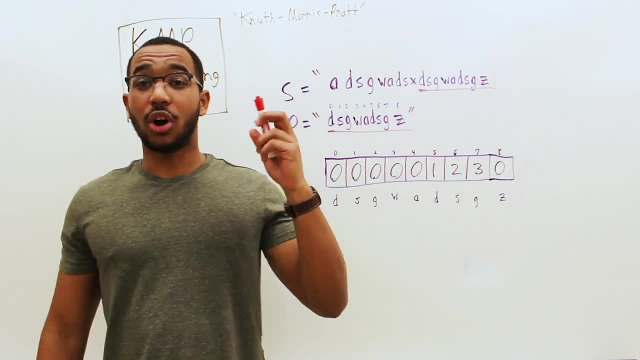 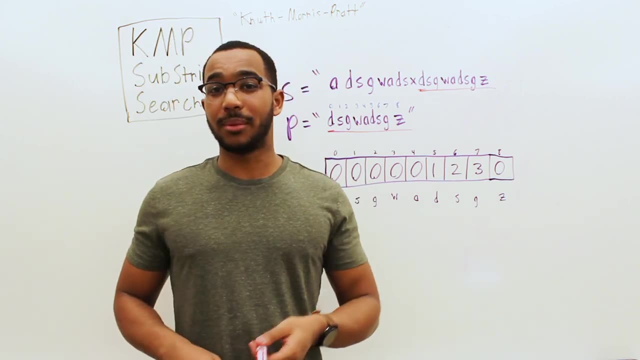 There's also Boyer Moore, Rabin Karp. These are other substring algorithms And these other linear time algorithms take different approaches. So let's do an algorithm analysis, a time analysis on this algorithm. So now let's look at each of the steps of this algorithm. 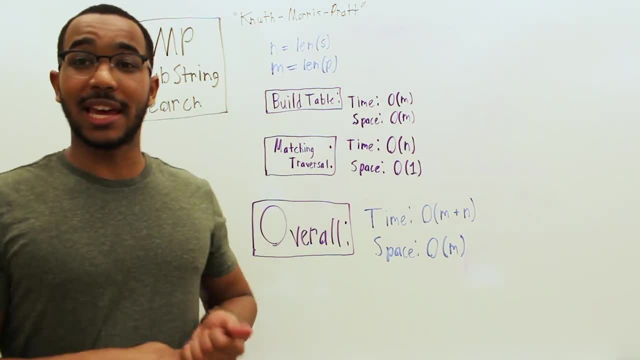 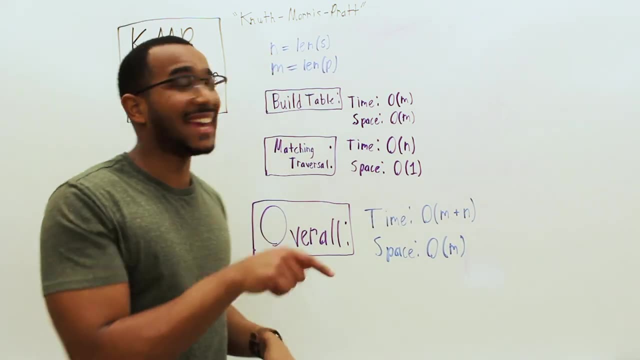 This algorithm consists of two basic steps, which is building the table and then performing the traversal with our table, N and M. We want to define them first. So N is the length of the string we're searching in, M is the length of the pattern we're searching for. 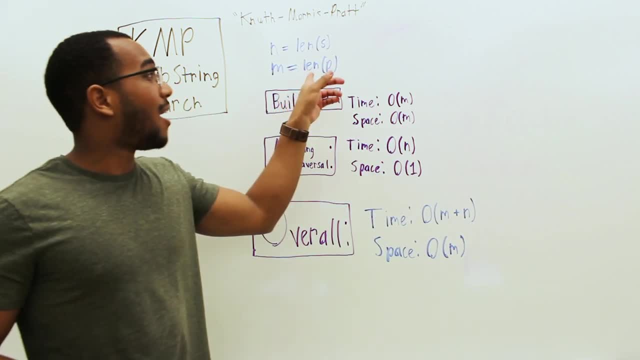 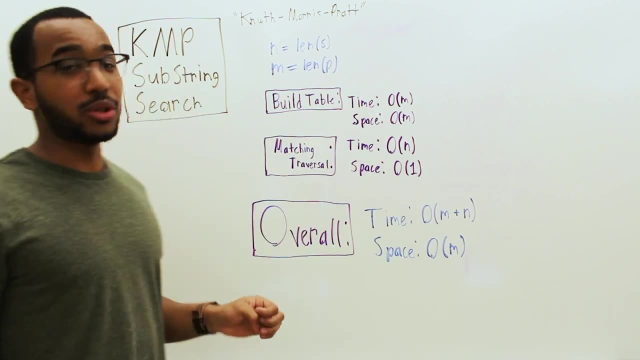 Building the table is going to take us the length of P time, which is going to be- we're just calling that M- the length of the pattern. So it's going to take us O time And it's going to take us O space. 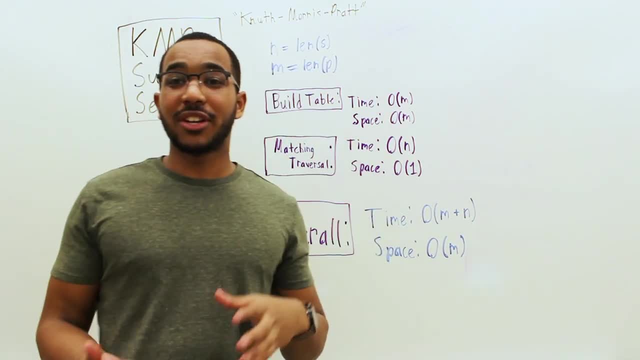 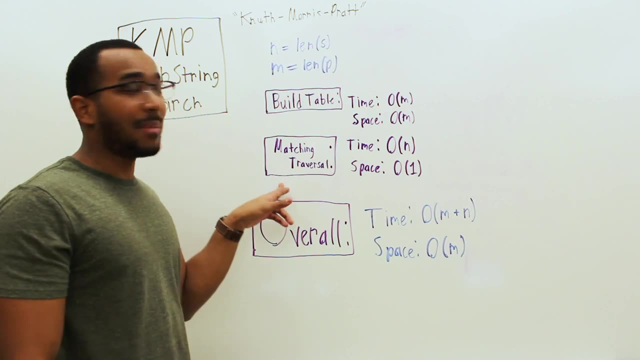 because we're keeping a track of the longest suffix. that is also a prefix up to that point for the pattern string. So that is the building table step For the matching traversal step. we're going to be doing O time. We're going to balance by O. 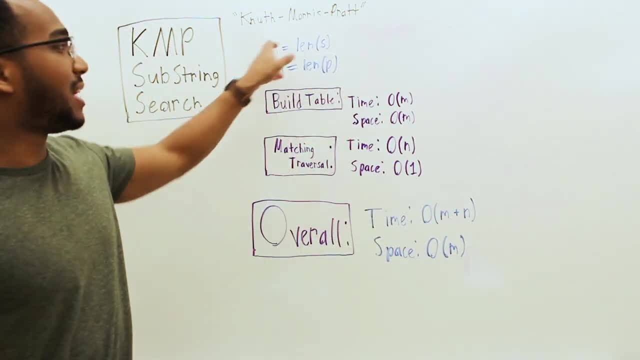 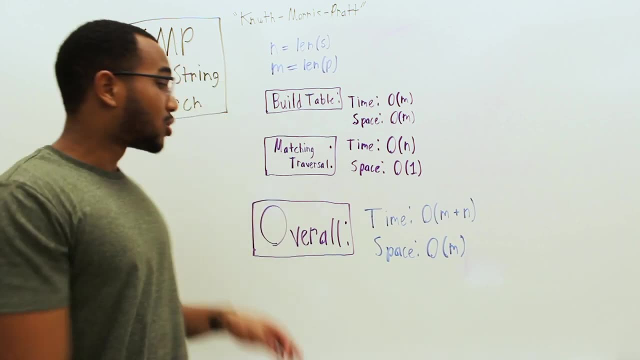 because that is the length of the string we're searching in. We define that up here And then the space is going to be constant because we're not creating any extra space. We're just performing comparisons during the traversal. So overall, this algorithm is linear with respect to each of our inputs. 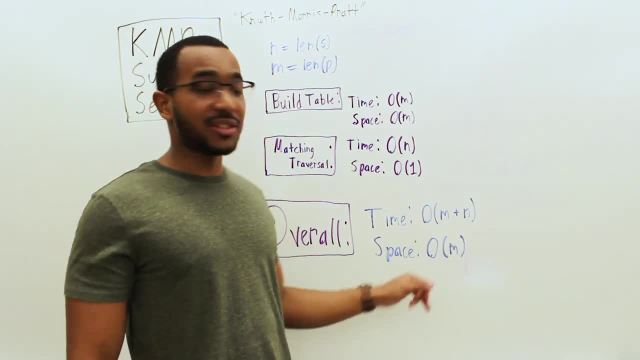 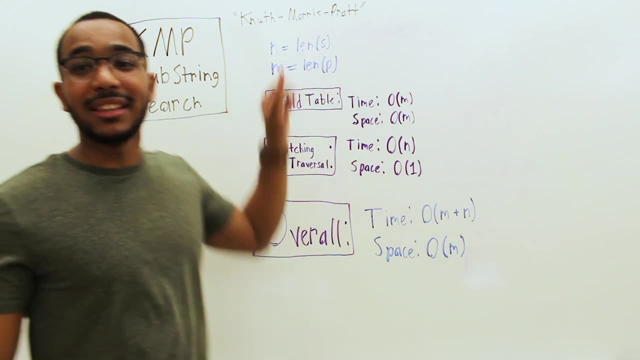 M plus N, we get O for time and we get O for the space. And remember: M is the length of the pattern, N is the length of the string we're searching in. So this is the KMP algorithm. This is actually not that bad to understand. 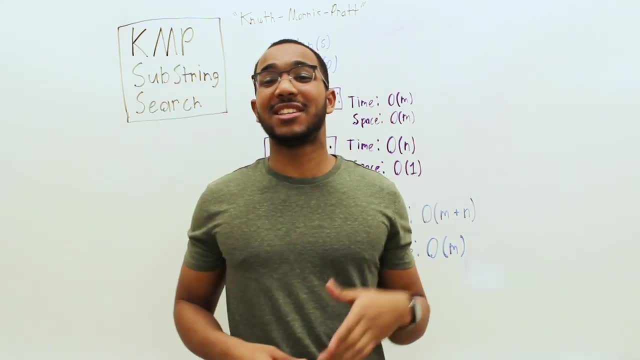 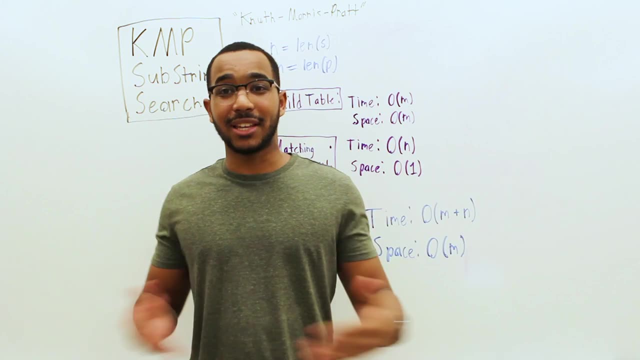 when you really understand why we look for prefix and suffixes, Why does that matter to us? So it becomes simpler when you understand that intuition and then from there it's just a matter of seeing the implementation in code. If you like this video, hit the like button.